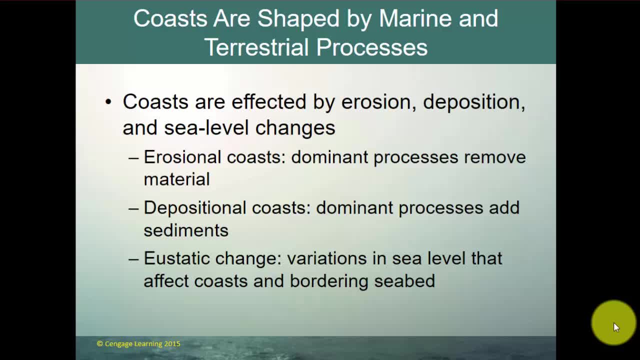 All right. How are coastlines shaped? Well, they are shaped by marine and terrestrial processes, not only what's happening with the ocean, but what's happening with land as well. Coasts are effected by erosion, of course, that's the movement away of sediment and deposition. the deposition or 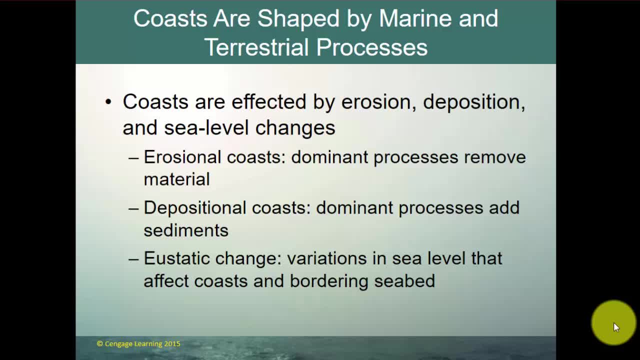 the placing of sediment and also sea level change, And sea level, as we have learned, has changed over all of geologic time. The thinking at this time is that generally, on a global scale, sea level is increasing and we can see, looking at different proxy data, that sea level has been increasing for about the last ten. 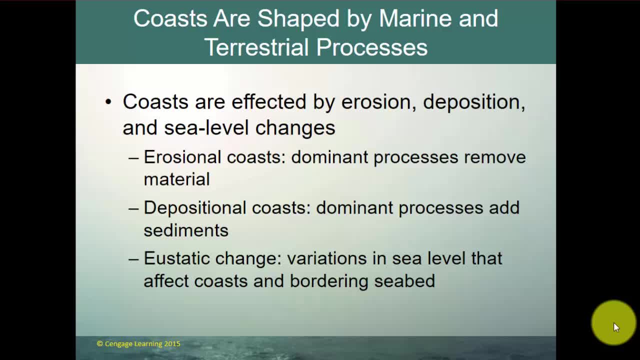 to eleven thousand years since the last ice age. the Wisconsin ice age ended. Erosional coasts dominate, dominant processes remove material and depositional coasts. the dominant processes add sediment and we talked about static change or again that concept of isostasy or isostatic rebound. 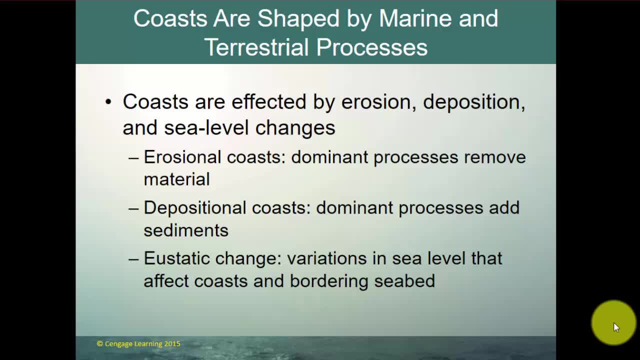 and that continents move up and down based on how much mass is in the continent. If more is added to the continent, it sinks and maybe sea level rises. If mass is taken away from the continent, it may rise and sea level drops. So those eustatic changes, variations in sea level that affect coasts and the bordering. 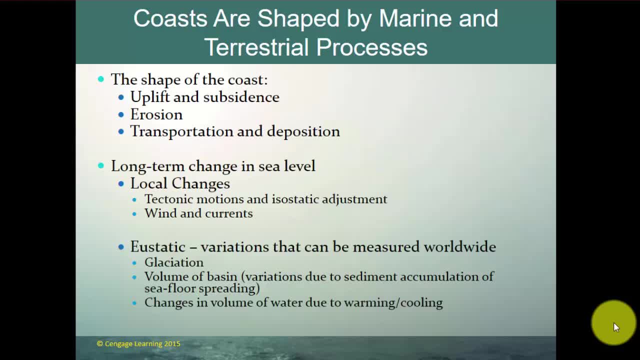 seabed. So the shape of the coast is a process, is a function of the processes of uplift and subsidence, erosion, transportation and deposition, Long-term changes in sea level. local changes can come from tectonic motions and isostatic. 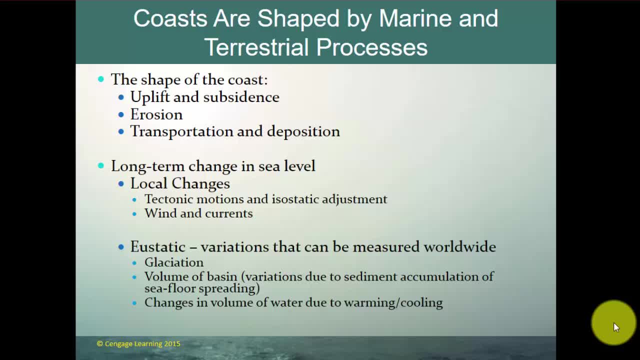 adjustment. There's also some coastal changes that can occur because of winds and currents and those eustatic variations that can be measured worldwide. Meaning: what is the sea level based on glaciation? Is there more ice locked up on the ice sheets and therefore less water in the ocean? The volume of a basin can vary. 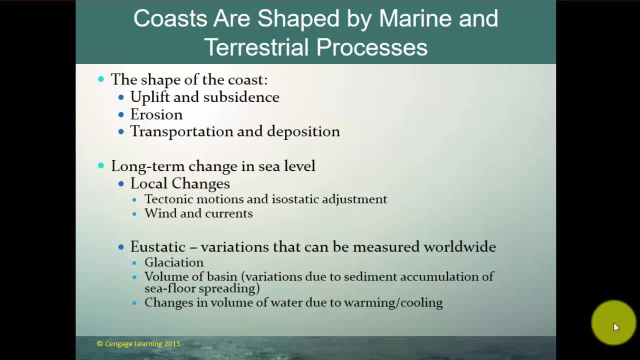 due to sediment accumulation, and also it can vary due to seafloor spreading. and we also see changes in water volume due to thermo expansion, Meaning a warmer sea surface is going to be thicker and a colder sea surface is going to be thinner. So all of these different processes at a global and at a local, 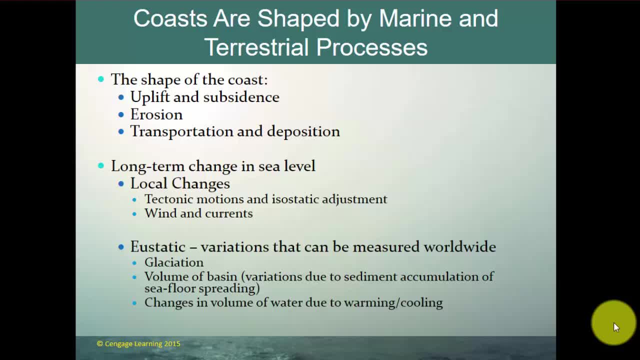 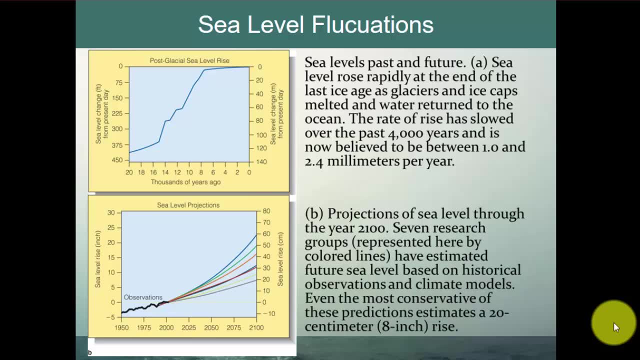 scale can change the shape of a coastline over geologic time. So let's talk about sea level. So let's talk about sea level. What we have known is that, again, essentially, sea levels have been on the rise for the last 10 to 11, maybe 12,000 years in a significant way. Sea 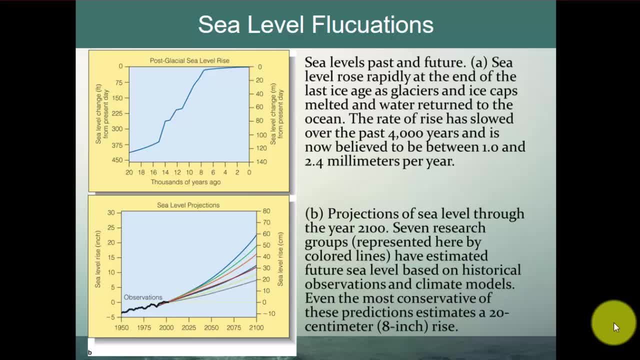 levels. past and future Sea level rose rapidly at the end of the last ice age as glaciers and ice caps melted and water returned to the ocean. The rate of rise has slowed over the last 4,000 years, is now believed to be somewhere between 1 and 2.4 millimeters per year, Although I can tell you that in the last 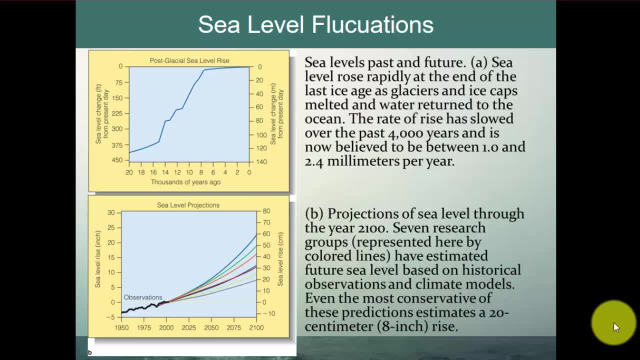 perhaps decade. since about 1992, a real attention has been paid to sea level rise and we're beginning to see from satellite altimetry and then also for just some tide gauges, that sea level rise being closer to 3, 3.5. 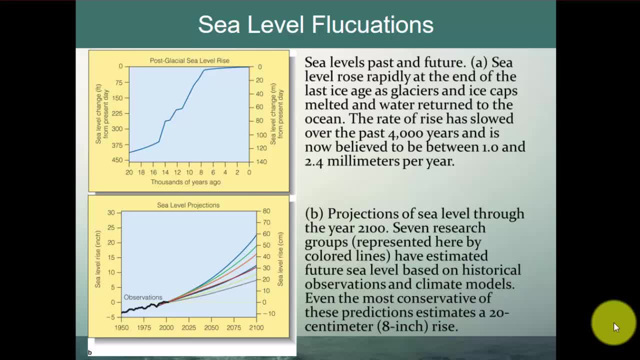 millimeters per year. So projections of sea level through the year 2100. and again you see numerous projections because there's numerous different models, but those projections- seven different groups have estimated future sea level rise, Sea levels based on historical observation and climate models, and even 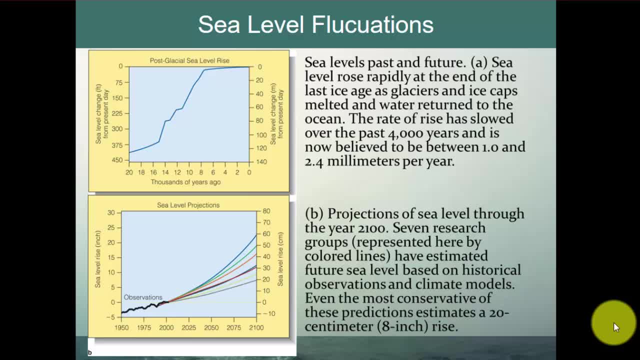 the most conservative of these shows a 20 centimeter or 8 inch rise. Some of the less conservative show a rise more on the order of two feet. so significant rises and again new data over the last 10 to 20 years has really begun to see. 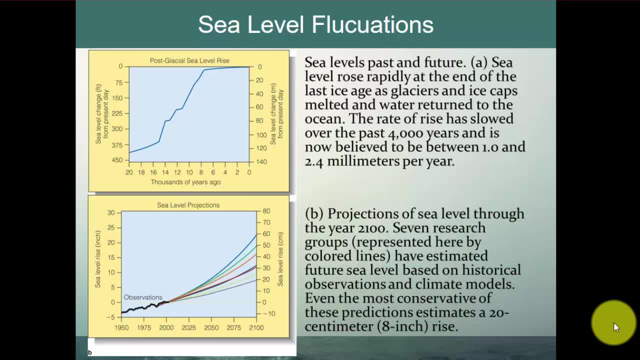 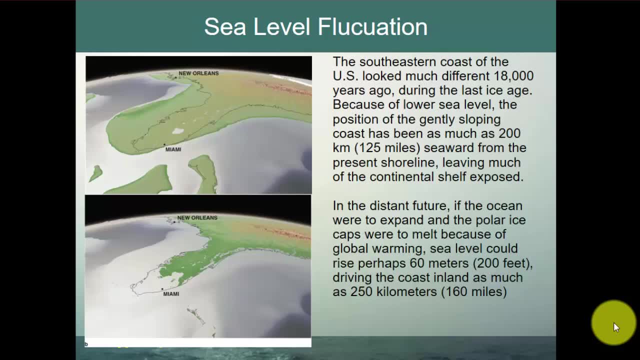 significant potential increases in sea level, and mainly from from two things: the melting of the ice sheets and then also that thermal expansion of the ocean As it does warm up. and so we know, looking at different types of sediments and deposits and cores, that the southern coastline of the US looked a lot. 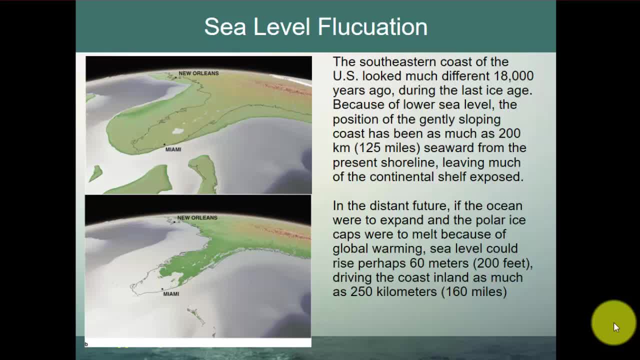 different. 18,000 years ago, The Florida Peninsula was much, much wider and it changed the climate. and this, this 18,000 year ago view, was because lower sea levels were in place due to the fact that most of the water was locked up in. 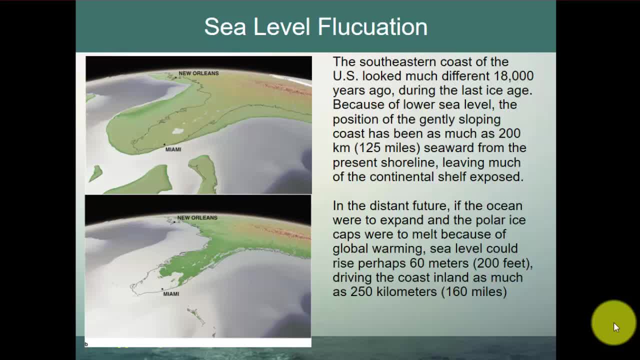 the ice sheets. So, because of lowering sea level, the position of the gently sloping coast had been as much as 125 miles further out to sea from the present shoreline, which meant that much of the continental shelf was actually exposed. Now, if sea level continues to rise in the distant future, 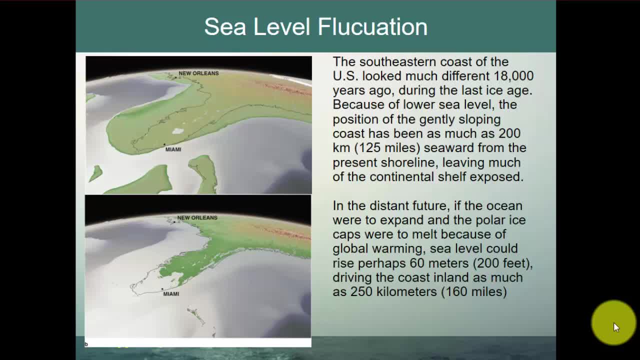 Florida could look something more like what you see in the bottom picture, but I will tell you that when we look at sea levels in the deep pass, we know that at times Florida was almost completely inundated or was completely underwater, and then in other times it was this very 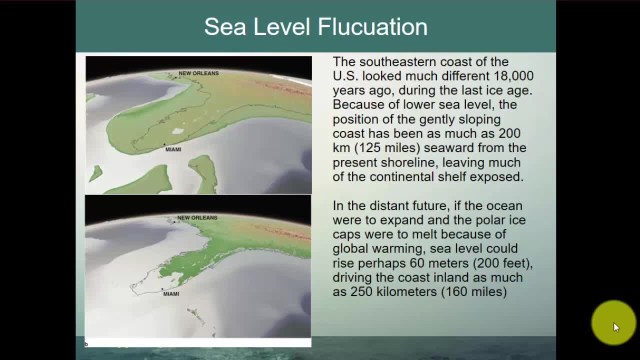 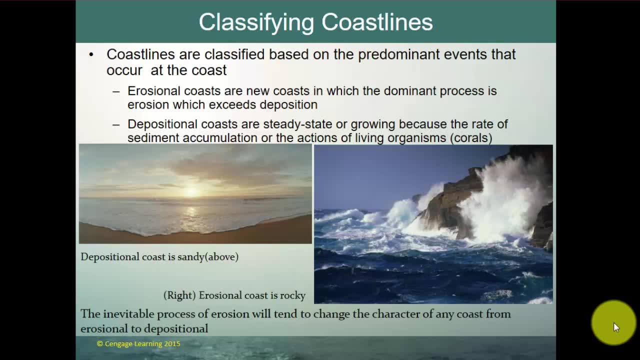 wide, broad peninsula, So there's been a lot of fluctuation- and what the state of Florida has looked like over the last 200 million years. So how do we classify coastlines? They're classified based on the predominant events occurring at that coast. Again, I've talked many times that science is all about classification. 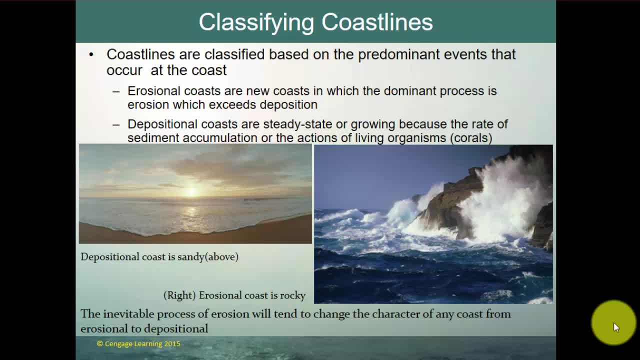 putting things in distinct groups. So erosional coasts are new coasts in which the dominant process is erosion, which exceeds deposition. Alright, more erosion is occurring than deposition. They tend to be rocky, and oftentimes they also tend to be coasts that are seeing a lot of. 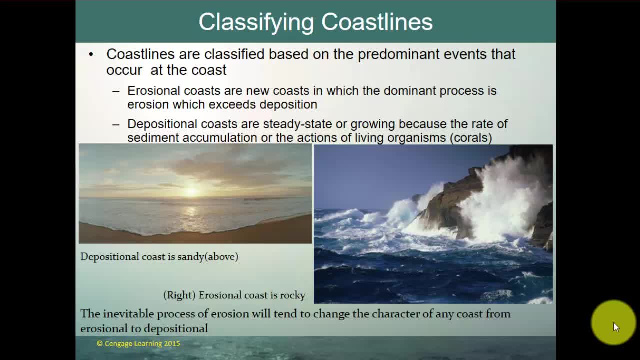 uplift. Depositional coasts are a steady state or sometimes they're growing because the rate of sediment accumulation is more than what's taken away, and sometimes it's also the actions of living organisms like coral. So you have a depositional coast in the picture where it's sandy and erosional coasts. 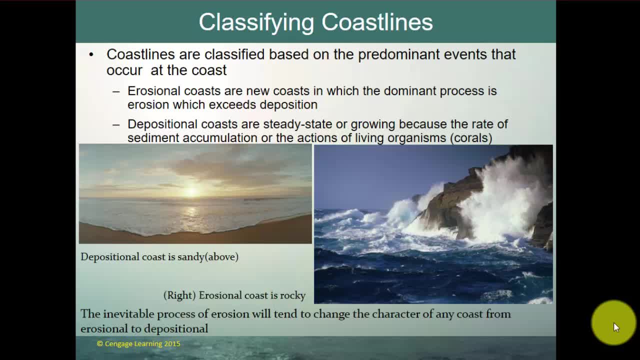 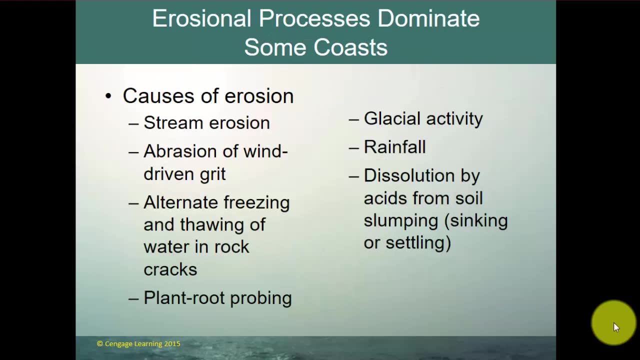 where it's rocky, The inevitable process of erosion will tend to change the character of any coast from erosional. So it starts out with uplift and erosion and rockiness, but eventually all that wave action will eventually change the character of any coast from erosional to depositional. So what are the causes of? 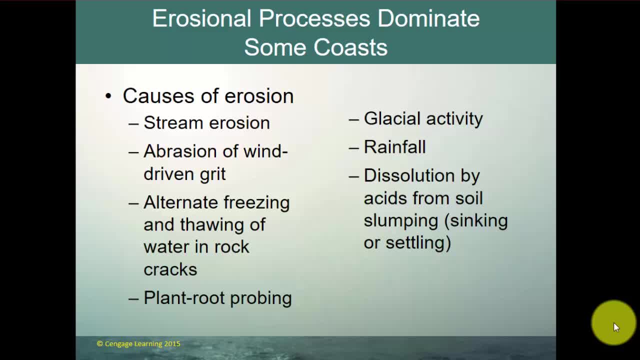 erosion: There's erosions from streams that flow in from the mountains. abrasion of wind: there's alternate and freezing and thawing of alternate freezing and thawing of water and rock cracks that help to break up rock. Plant roots can weather and break down rock. Glacial activity can. 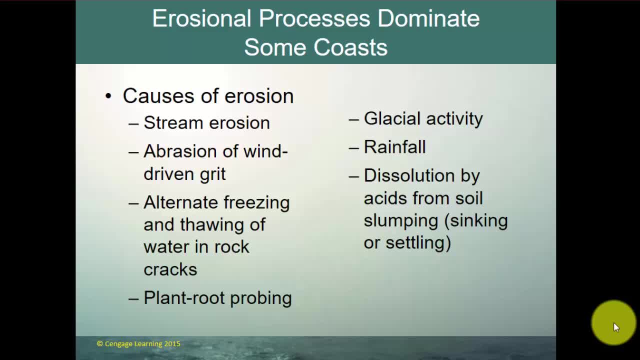 create erosion. Rainfall can create erosion- Dissolution of acids from the soil, which includes sinking and settling Lots and lots of ways that you can that that rock can be broken down by weathering and then eroded. Now much more detail is given to this concept in an earth science class and and as part of 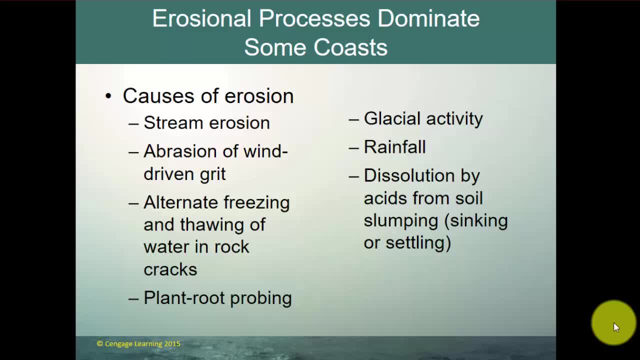 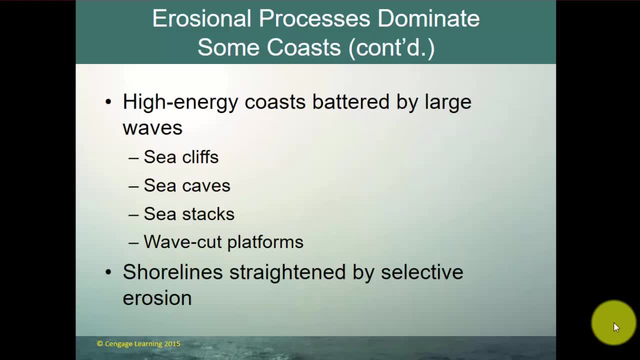 your science curriculum. you may want to consider taking an earth science class and talking more about erosion and deposition and how it works. So high-energy coasts are battered by large waves. High-energy coasts tend to have sea cliffs and sea caves and sea stacks and wave cut platforms. 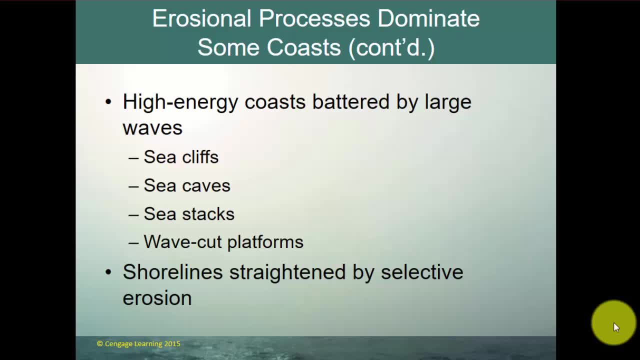 Eventually, even those high-energy coasts begin to be straightened out and also changed into less high-energy coasts and more into depositional coasts, as selective erosion can occur And literally what can be rocky and jagged coastlines can be straightened out over many, many thousands, or maybe hundreds of thousands or close to. 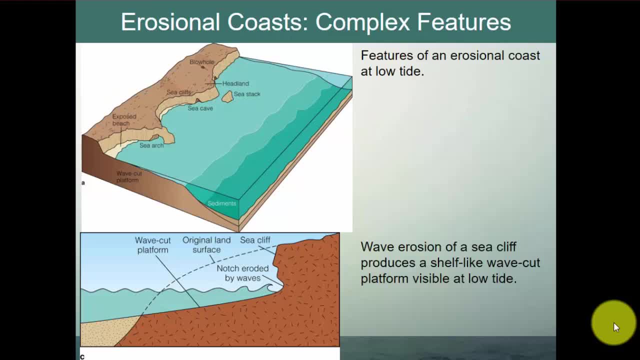 millions of years. So here's your erosional coast at low tide. We've got your sea arches, your sea caves, your big cliffs, your sea cliffs, your sea stacks. And as that water moves up, it erodes and breaks away the sea cliff and 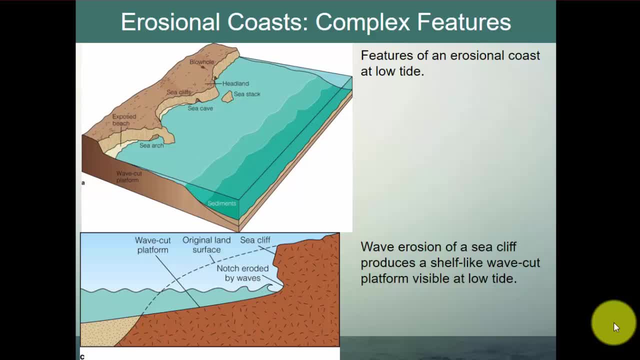 what ends up happening is below the level of the water. you get these wave cut platforms. So the wave cut platform is going to be very, very flat. Wave erosion of the sea cliff produces a shelf life wave cut platform. Typically, it's only going to be visible at your low tides. So here's the result of wave action on a 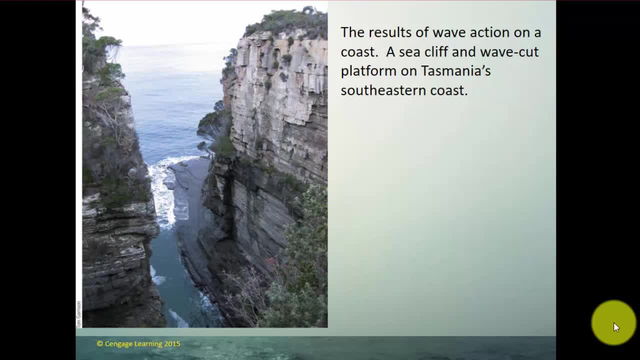 coast. You see these deep sea cliffs and that wave cut platform. That's what you see between the two cliffs, That flat like table, like structure there. That is a wave cut platform. That's Tasmania, which is, of course, the island south of Australia, and this is, of course, is going. 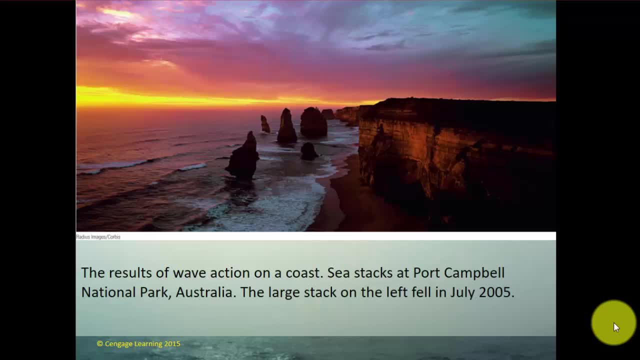 to be at low tide. All right, here's another sea stack. This is another thing where selective erosion or just differences in the way the waves strike the coastline breaks off these sea cliffs and leaves these sea stacks. Now, eventually, those sea stacks will be eroded away as well, and you can already. 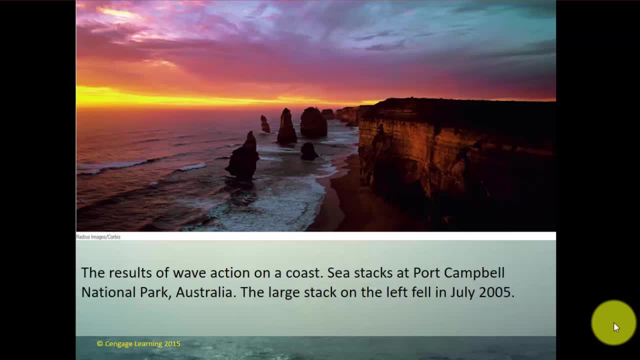 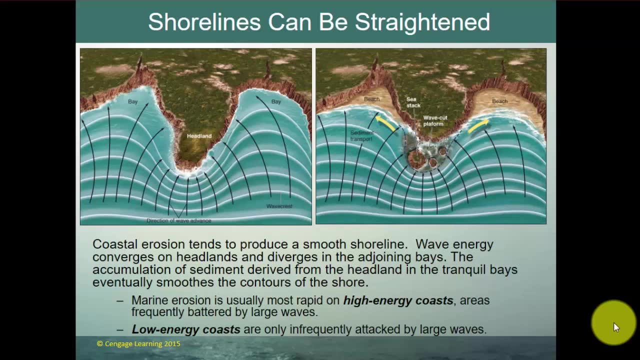 see how this coastline is going to be eroded away. So you can see how this coastline is going to be eroded away as well, and you can already see how this coastline is beginning to be straightened to some degree. and this is another photograph from Australia. So this is how that selective erosion occurs: Coastal erosion. 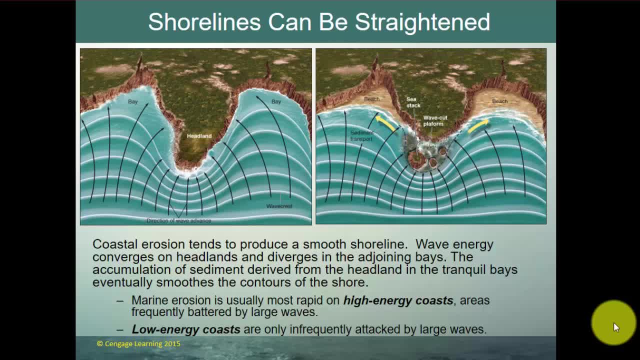 tends to produce a smooth shoreline, So shorelines are smoothed out and straightened by coastal erosion. Wave energy converges on headlands- Again, we're going to talk about refraction of waves- but it tends to bend them into headlands and so you get wave energy focusing on both sides of the headland and 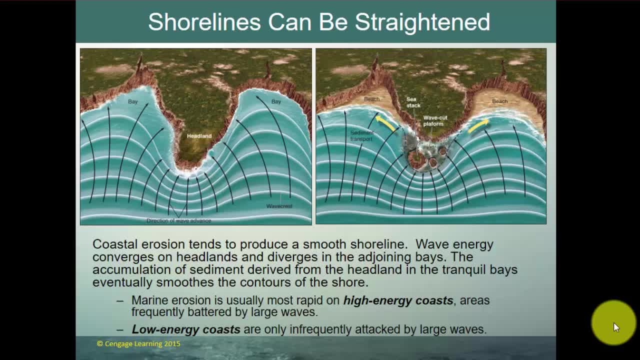 then it tends to be less in the, in the bays. So the accumulation of sediment derived from the headland and the bays eventually smooths the contour of the shoreline. So you can see, a headland eventually turns into these sea stacks and as those beaches deepen and thicken, the entire coastline straightens out. So 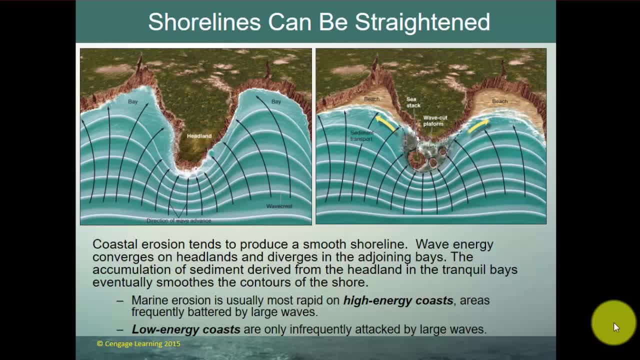 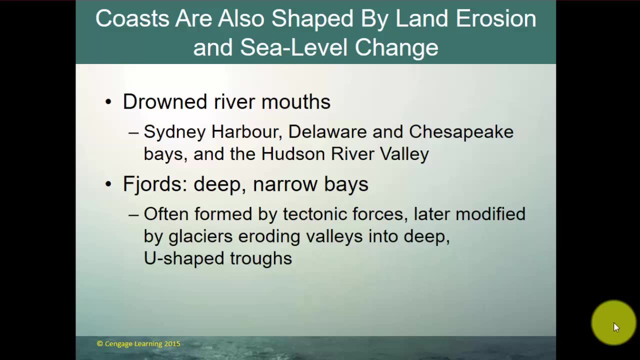 marine erosion is usually most rapid on high energy coasts, frequently battered by large waves. Low energy coasts are only infrequently attacked by large waves, So coasts can also be shaped by land erosion and also sea level change. So sea level change may actually cause sea level to rise up into what used to be. 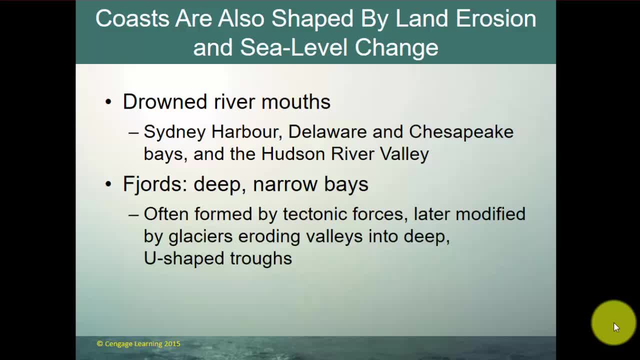 some deep canyon or where a river has cut down to the sea, and in those situations you get what are referred to as drowned river mouths. So we talked about Sydney Harbor, but much better examples of drowned river mouths are the Delaware and the Chesapeake Bay. 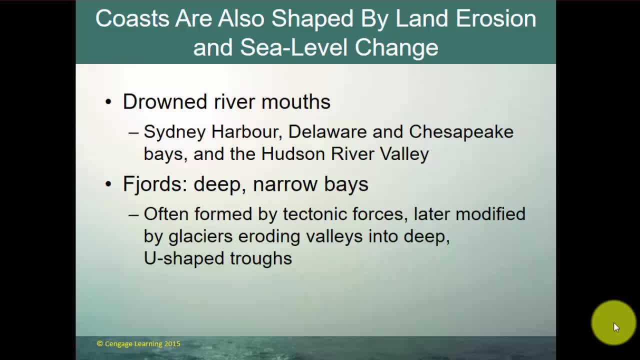 And the Hudson River Valley, where sea levels have come up and literally drowned old rivers that had cut down through the continent. And then fjords are deep, narrow bays and they're also formed by tectonic forces and later modified by glaciers that that moved down and eroded the valleys into deep u-shaped troughs, and 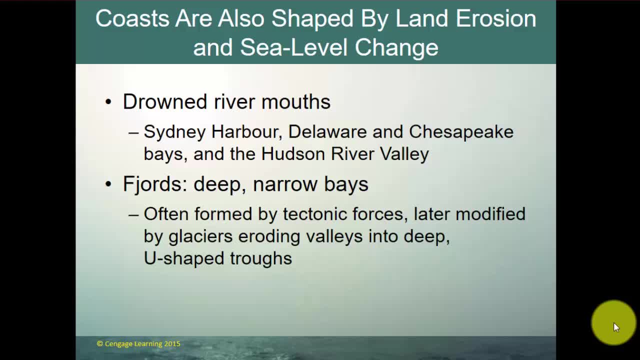 then, as sea level comes up, it drowns those u-shaped troughs and you get these deep, narrow fjords. So we'll talk a little about beaches, We're going to talk a little bit about lakes, we're going to talk about the. 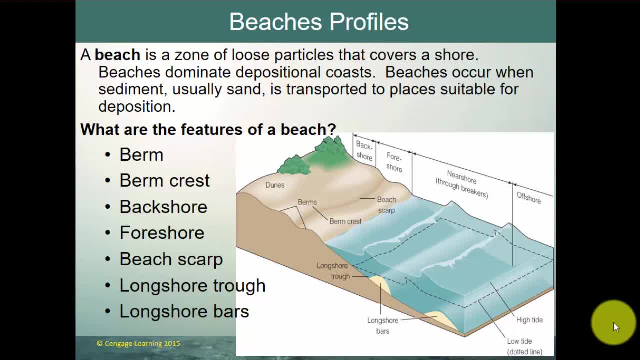 And we'll talk a little bit about beaches. we're going to talk about the. we'll talk a little bit about beaches. we're going to talk about the showed you how sea cliffs can be eroded away and beaches develop in the more tranquil bays, and so a beach zone, or a beach, is a zone of loose particles that. 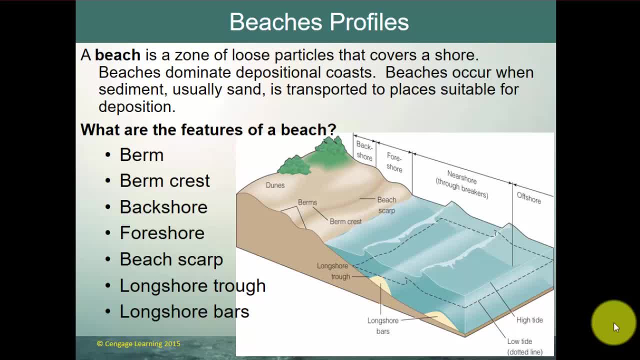 cover a shore, beaches dominate depositional coastline. so when it's erosional you're seeing the uplift and the battering, but as that the character changes to a depositional coastline. that's when you start to get beaches. and beaches occur when sediment, usually sand, is transported to places suitable for. 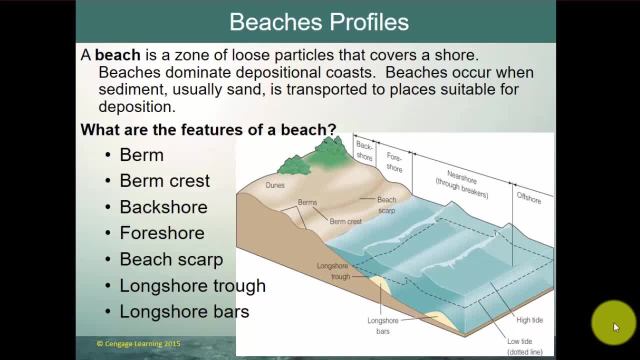 deposition, meaning it's moved there and then it's able to fall out of the median, moving it mostly water, sometimes wind, and be stable. so we have some unique features of the beach, including the berm, the berm crest, the back shore, the foreshore, the beach scarp, longshore trough and the longshore bar. so the 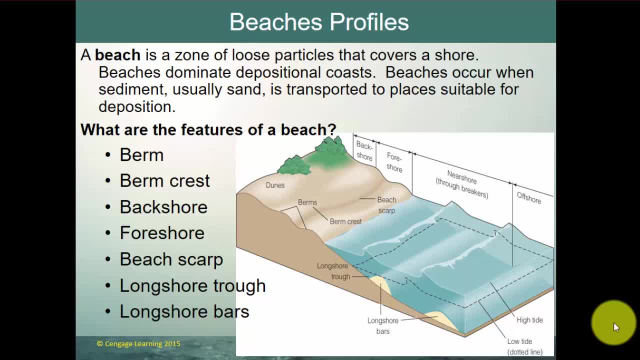 back shore is what's going to be up against the dunes and the foreshore is going to be what separates the back shore from the actual water itself. the near shore is going to be a those the breakers, and the offshore is just out beyond where the breakers are. 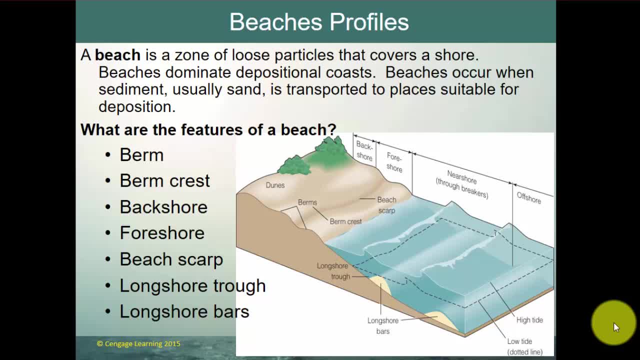 and the wave action tends to create these burns and berm crests along the beach and beach scarfs, and the beach scarf is where maybe high tide comes up to and so it erodes away up to that point and that leaves a little bit of a 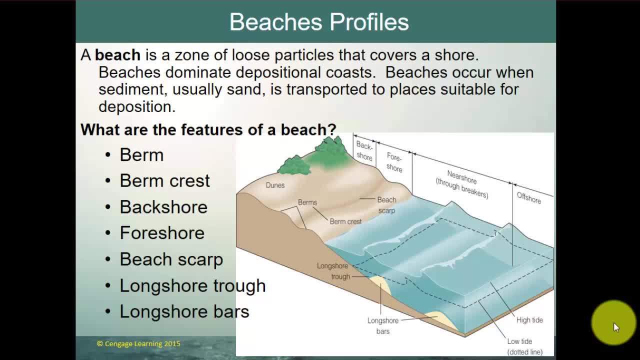 small cliff in the sand and you've seen that at our local beaches. at times in the summertime you don't see it as much as you see it in the wintertime, and then the way water pulls sand back off the ocean, you tend to get these longshore. 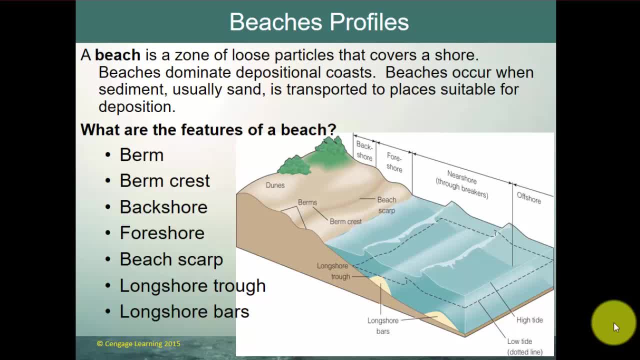 bars, and these longshore bars are the ones that are the most likely to get damaged and smaller, and there's some things that get damaged. cleanup rings are very important because if you listen to media talking about beach and boating conditions, oftentimes I want to talk about the young, the rip, current threat and rip. 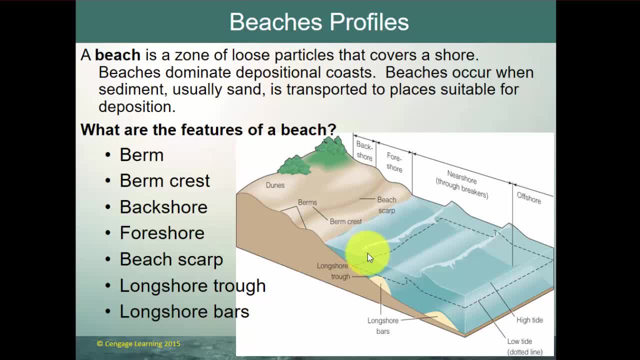 currents literally occur where these longshore bars are cut out by waves. and when we talked about waves, we talked about longer period waves, being able to feel the bottom earlier. so if you have a very short period wind wave, these waves just sort of move over these longshore bars and break onshore. but it gave him a. 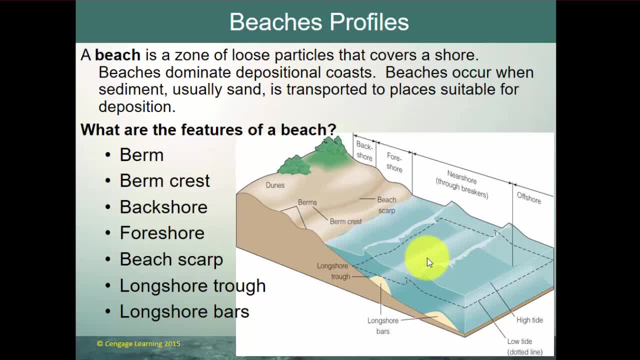 much longer period wave that feels the bottom earlier. those waves get soft and those wave circles, those epi circles, will will tend to erode and break out these longshore bars, and so what happens is you get a bar that's sustained and then an area where it's broken. 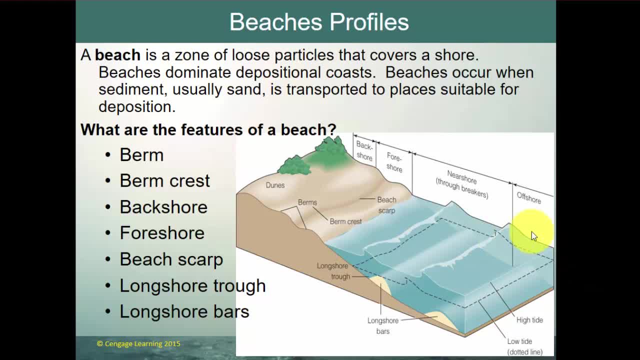 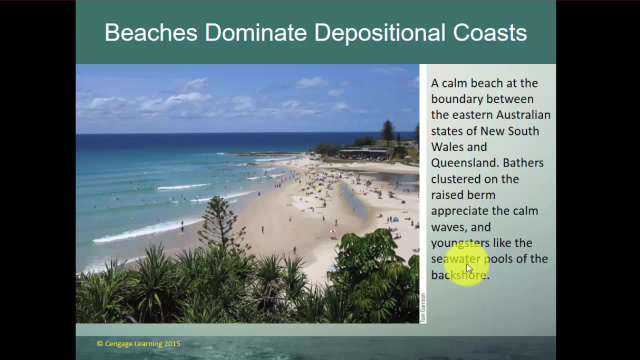 out because of a longer wavelength of waves, and what happens is water gets pushed up the beach and tends to rush out, and that break, and it's in that break, in the longshore bar, where you tend to get your rip currents, all right. so, um, depositional coastline, low energy, this is a you know what. 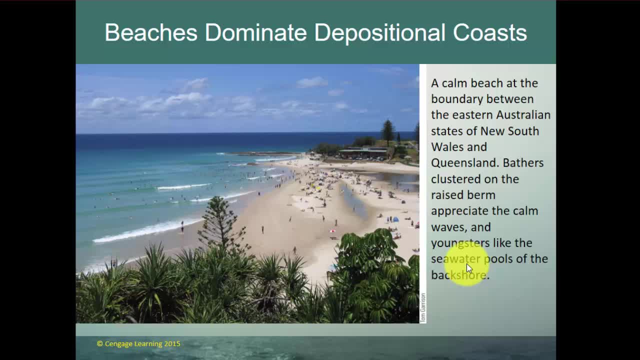 basically think of at the beach, and this happens to be yet another picture from australia, but you can see that you've got calm, waves and seawater that pools in the back shore and it's a very, very calm and settled environment and that's going to be a depositional coast. your erosional 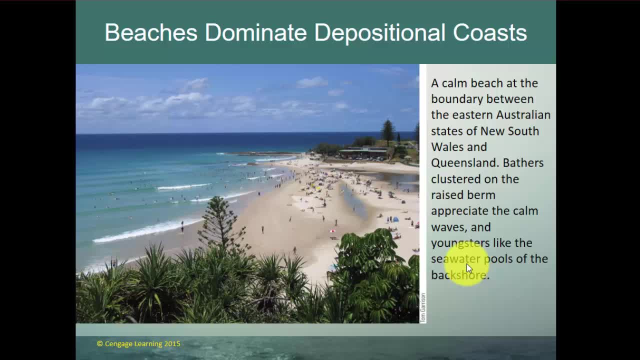 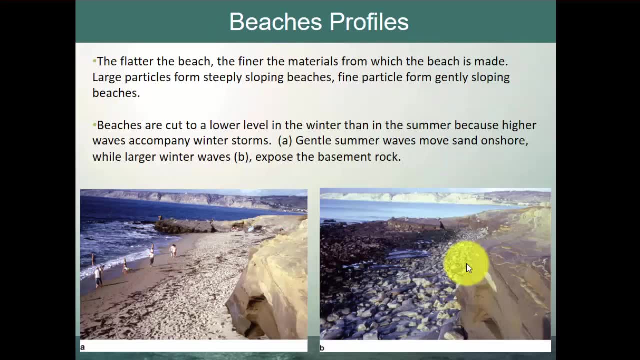 coast is going to be: the cliffs and the battering, breaking waves, a lot like what you see in parts of hawaii, a lot what you see in california and the new england coastline north of boston. all right beach profile, flatter beaches. the flatter the beach, the finer the material from which the beach is made. so 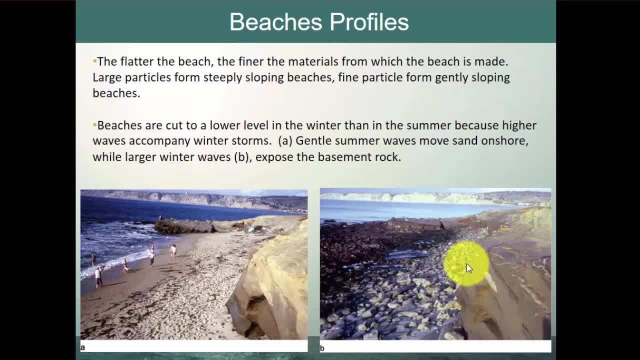 if you have very, very fine powder sand beaches, you tend to get nice wide beaches, and we think about that on the gulf coast, particularly some gulf coast beaches on the panhandle, where you have more larger particles. you think of the beaches you might see on the east coast or even 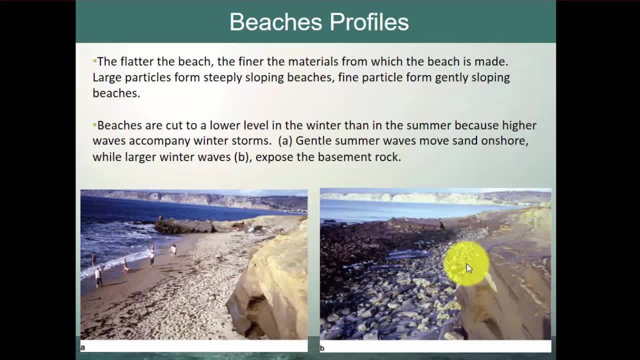 down in the key. so the flatter the beach, the finer the materials from which the beach is made. large particles tend to form the beach and that's what we're talking about here. so you're going to see, there's a lot of steeply sloping beaches and fine particles tend to form. 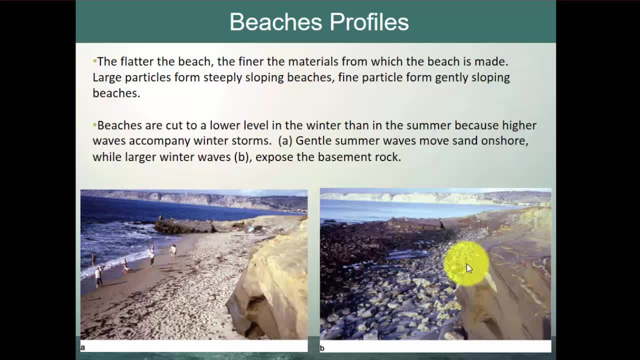 gently sloping beaches. now, beaches are cut to a lower level in the winter time because of more wave energy. winter time tends to have more storms and more waves, and then gentle similar ways. summer waves tend to move sand onshore, while larger winter waves tend to pull sand offshore and 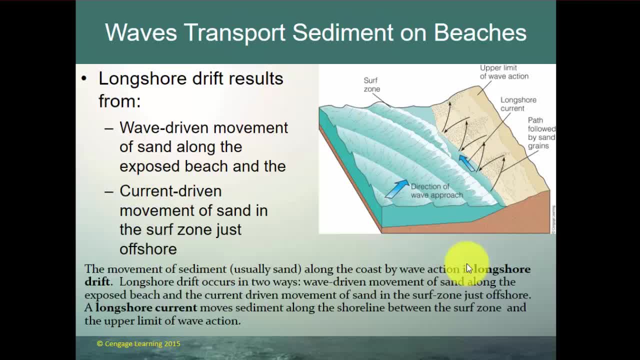 expose that rock at the basement. all right, longshore drifts: these are bad weather conditions. they tend to get a little more heaty. now that we've seen the sand go hard and it's starting to get shore Predator that we've been talking about and that's kind of going along with the sea and the water is going to go down this side of the river and 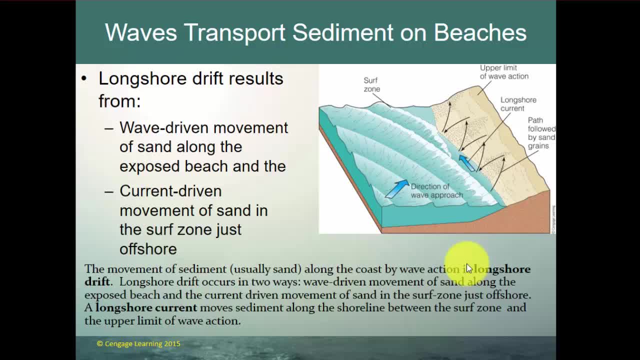 the water is going to go down that side of the river, so that's going to make the most damage that we can get so this time. so wind-driven movement of sand along an exposed beach and the current driven movement of sand in the surf zone just offshore creates what's known as long 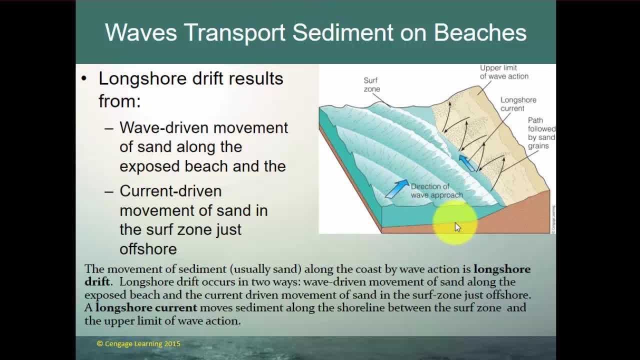 shore drift and essentially the waves are going to come in at an angle and the sand is going to move up with the water and then the move comes straight back down. so you basically are taking sand from here and moving it up the beach and then it comes back down and sand from here up the beach and comes back down. 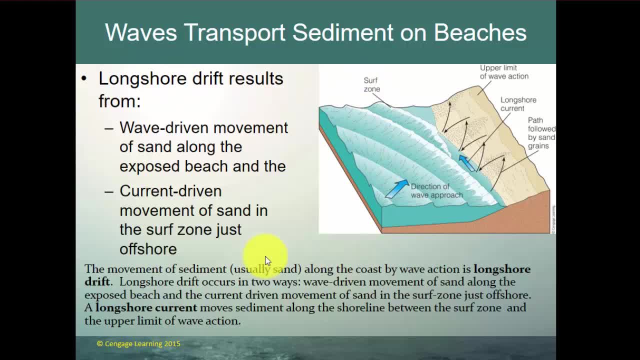 and in the end you tend to create this long shore drift. the movement of sediment, usually sand, along the coast by wave action is called long shore drift. long shore drift occurs in two ways: wave driven movement of sand along the exposed beach, which I just described, and the current driven movement of sand in 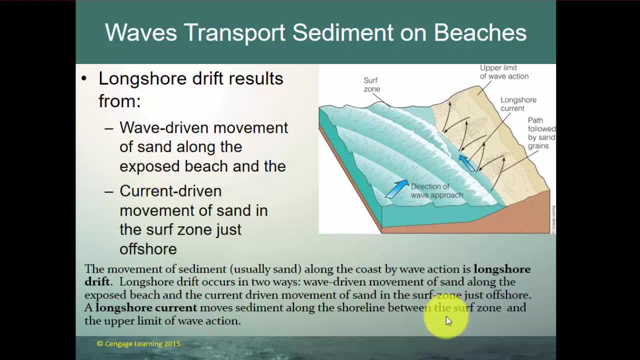 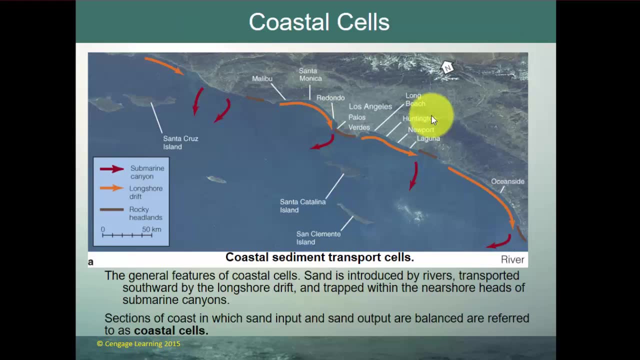 the surf zone. so this is the current moving sand up the beach. the longshore current moves sediment along the shoreline between the surf zone and the upper limit of wave action. so from about here back to about here, sand is moved and that is that longshore current all. 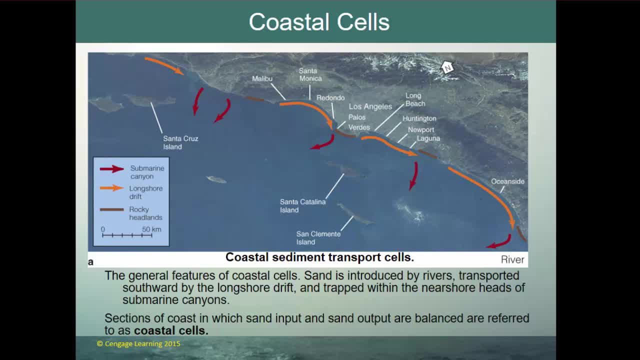 right, we're going to talk a little bit about coastal cells and how coastal sediment is. it's moved within a coastal cell, so I've got a couple of pictures here. you got the red lines or submarine canyons. that's going to be where maybe a 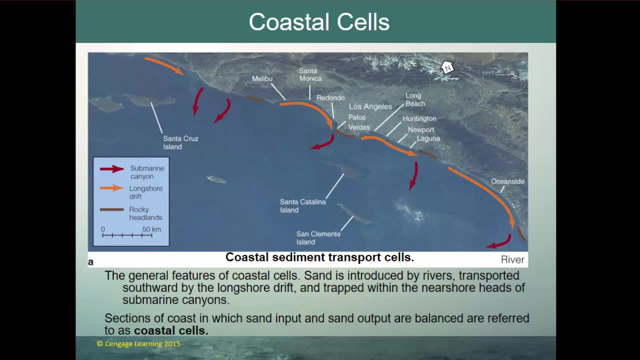 river comes out and cuts a valley in the land and then also a canyon on shore, and then you got your longshore drift, which you talked about, the drift of sand along the coastline, and then you can see we have rockier headland. so the general features of coastal cells, sand is. 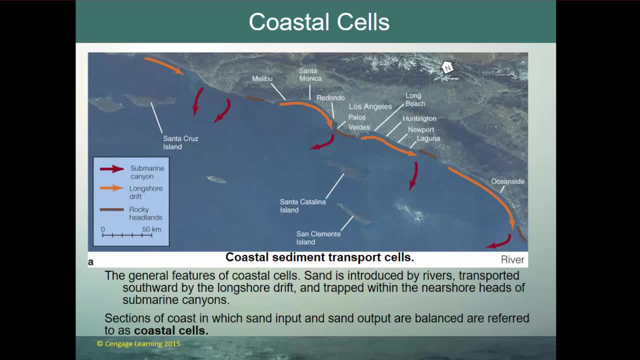 introduced by rivers and then transported, in this case, southward by the longshore drift and then trapped within the nearshore heads of submarine Canyon. so a section of coast in which sand input and sand output on our balance is referred to a coastal cell. it's an area where there's enough coming. 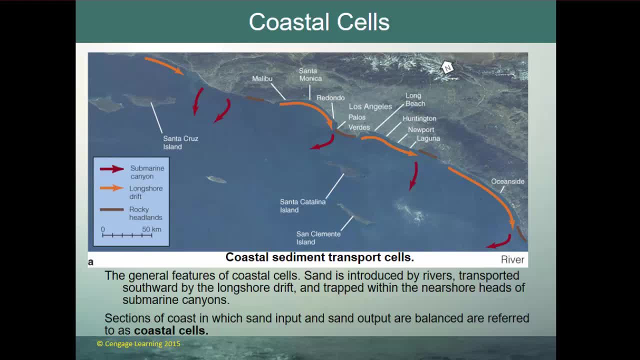 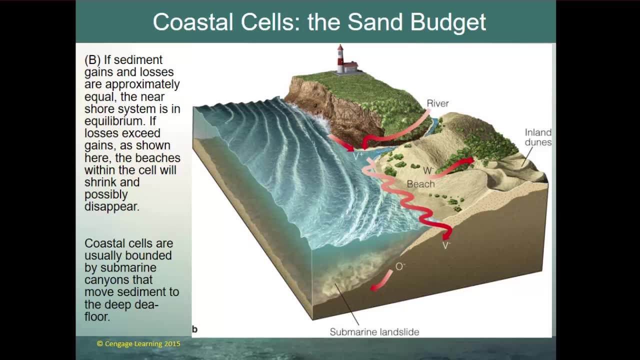 in enough, going out that the entire thing remains in balance. that's going to be your coastal cell. if sediment gains and losses are about equal, the near shore system is in equilibrium. if losses exceed gains, as shown here, the beaches within the cell will shrink and possibly disappear, so you can. 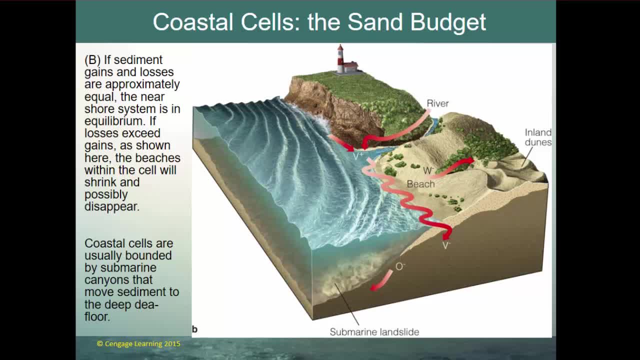 see in that where you have that river, you're getting sand coming down and it produces beaches to the south. but if there's less coming in than is being taken away, those beaches will disappear. coastal cells are usually bounded on either side by submarine canyons that move sediment. 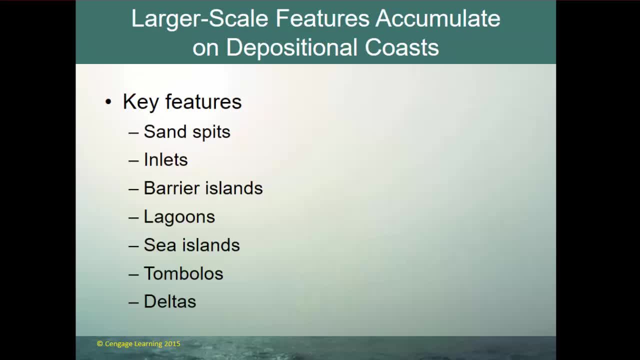 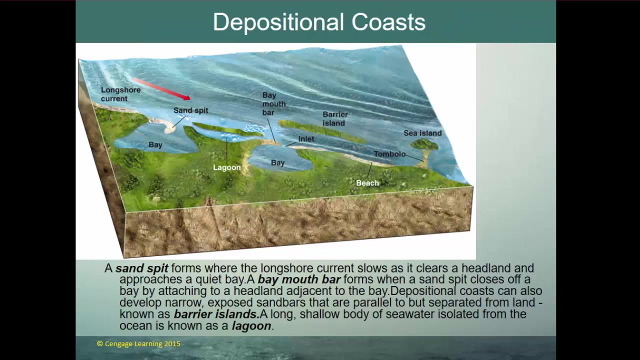 to the deep sea floor. all right, let's talk about the larger scale features that accumulate on a depositional coastline. so florida, the southeast, is a depositional coastline. some of the features that we have are sand spits, inlets, barrier islands, lagoons, sea islands, tombolos and also deltas. so here's a kind of the view of all of those things. 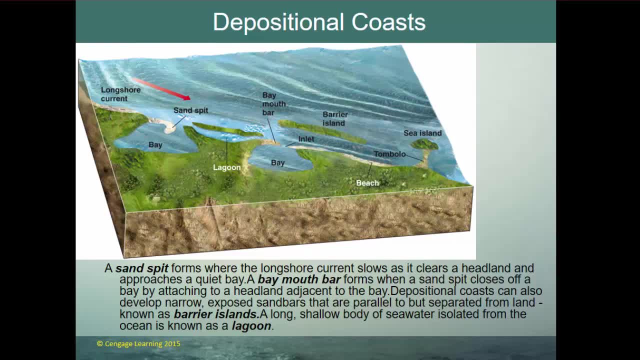 the longshore current is going from left to right in this picture and because it's going to move sand from left to right, you're going to have a couple of interesting features. first off, that longshore current in the upper left corner pulls sand across that open bay and eventually a sand. 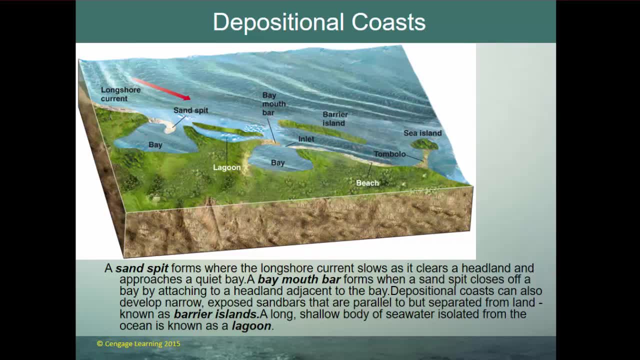 spit forms. now a little bit further down to the second bay, you can see where that sand spit has developed in what's called a bay mouth bar and it's almost closed that bay off and there you have an inlet. you also see where sand moving down the coastlines create a barrier island. 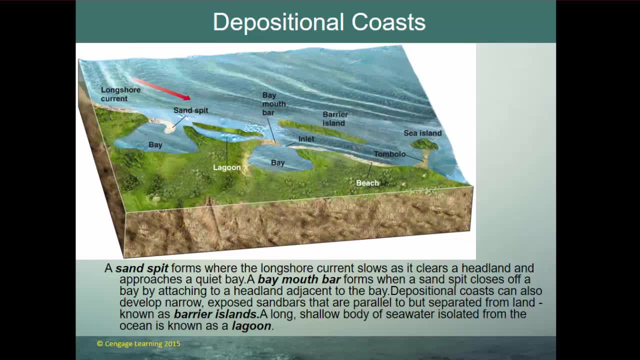 the one barrier island has also created a lagoon and then where there's a sea island offshore, a little tombolo has formed where sediment drops and creates a little land bridge from the coastline out to the sea island. so sand spits form where the longshore current slows as it clears a headland. 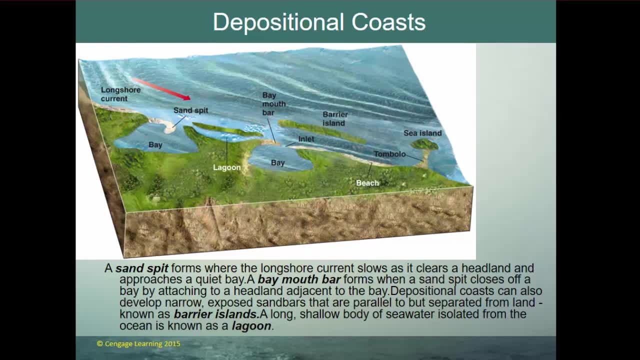 and approaches a quiet bay. so when the water slows down the sediment falls out. a bay mouth bar forms when a sand spit closes off a bay attached to a headland adjacent to the bay, so the bay mouth bar is where it just completely closes off the bay. depositional coasts can also. 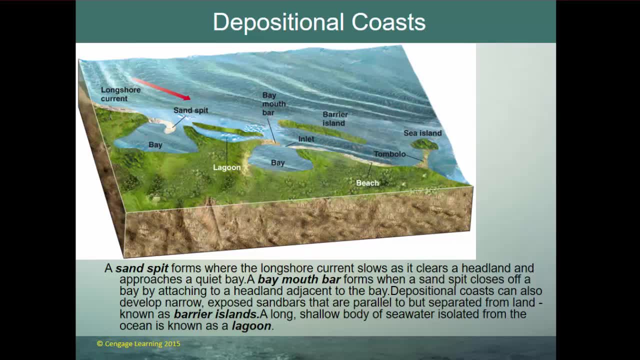 develop narrow, exposed sandbars that are parallel but separated from land, known as barrier islands, and the long, shallow body of seawater isolated from the ocean is therefore then known as a lagoon. barrier islands, then, are narrow, exposed sandbars that are parallel but separated from the land. 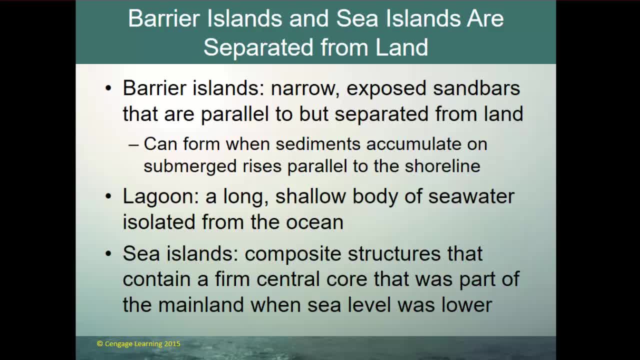 they can form when sediments accumulate on the submerged rises parallel to the shoreline. so those those longshore bars, if they get big enough, they can create the barrier island. the lagoon develops back behind the barrier island, a long, shallow body of seawater isolated from the ocean and then sea. 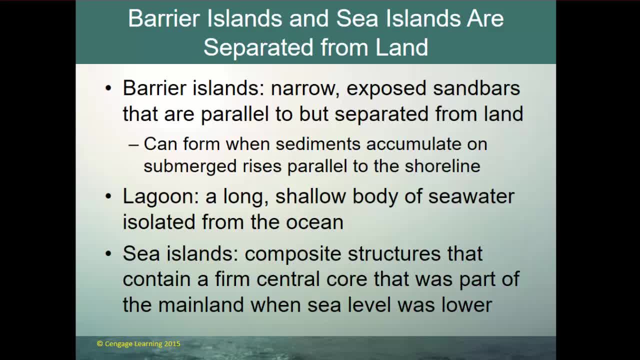 islands somewhat different. they're composite structures that contain a firm central core that was part of the mainland when it was built, when sea level was lower. so essentially, a sea island is going to be where, when sea level was lower, it was actually part of the mainland, but as water came up it drowned all the land around. 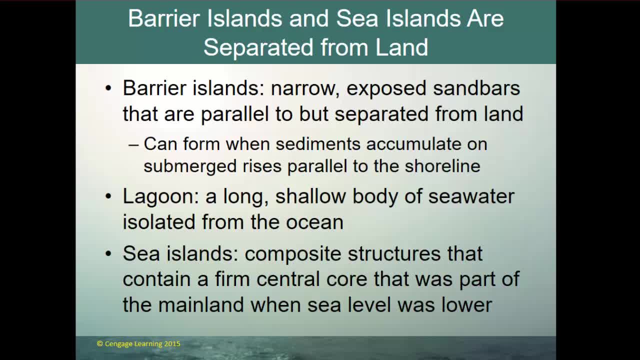 it and just left the sea island, so it's got a strong scent rocky core. essentially that holds the sand in place. now going back to the barrier islands. barrier islands are are those exposed sandbars and if they get anything that grows on them that puts down roots, it helps to hold the 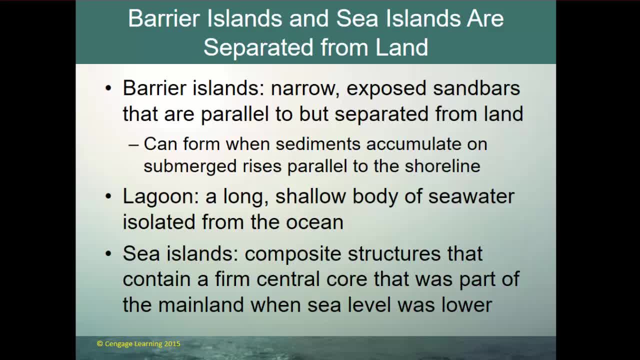 sand in place and barrier islands form. but the natural process of a barrier island is it to four of them is to form offshore and then, over a period of time when large sea waves occur because of storms, the sea waves will actually wash over the barrier island, moving the sediment from the front. 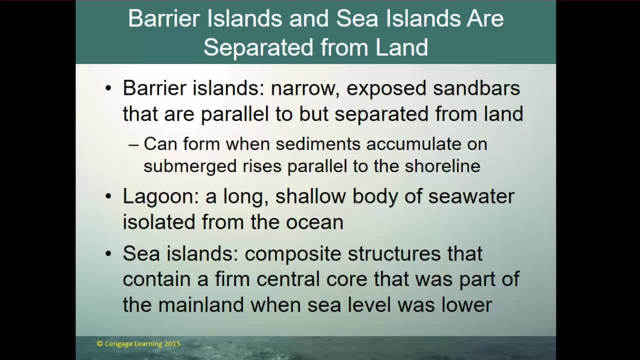 of the barrier island, the back of the barrier island, and in that way, barrier islands that are not developed are actually will migrate back toward the coastline, and we can see that along the east coast of the united states in areas where we have developed barrier islands and put up sea. 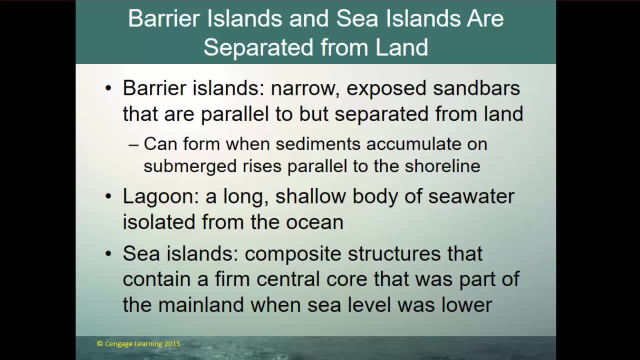 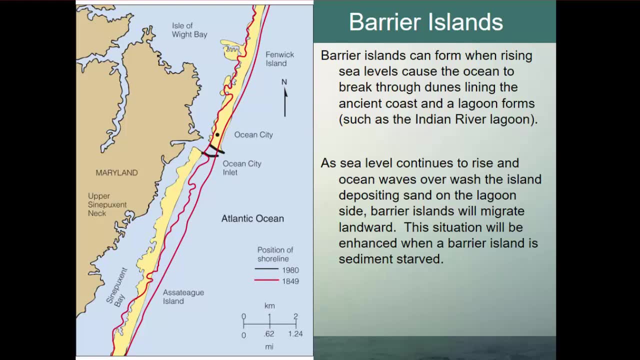 walls and put up jetties and whatnot, the barrier islands stay still, they're static, it doesn't move. but bear islands that have not been developed, they'll actually move toward the coastline, and that's the natural process of a barrier island, and so that's the way that look. this is something specifically that's happened in maryland with 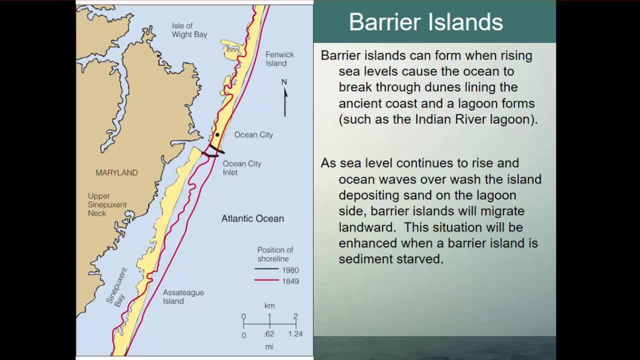 the ocean city island barrier island's been developed and the island to the south of it hasn't been developed and you can see where the position of the shoreline was in red in 1849 and when this particular study was done in 1980, how far that that southern island had moved because of the national processes. so the 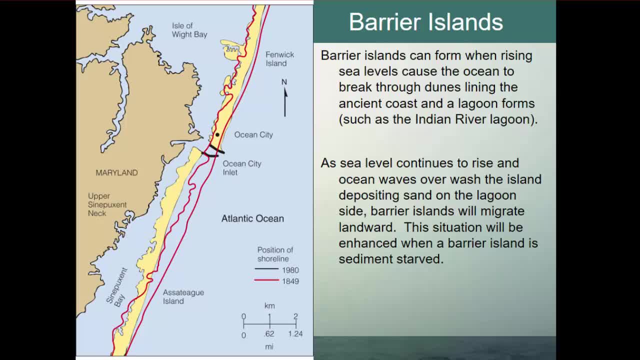 natural processes the barrier islands can form when rising sea levels cause the ocean to break through dunes, while in the ancient coasts and lagoons form, such as the indian river lagoon, as sea level continues to rise and ocean waters wash over the island, depositing sand in the lagoon. 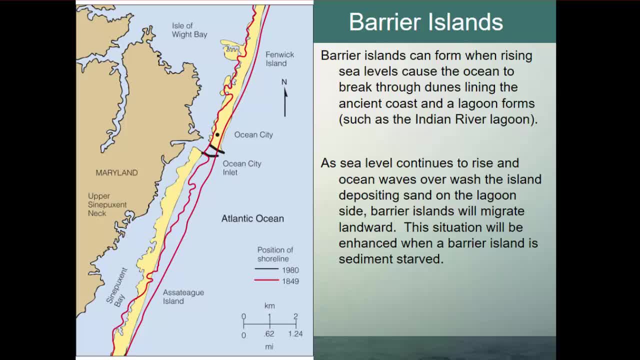 barrier islands tend to migrate landward, and this situation can be enhanced if the barrier island is sediment starved. and so, because of the, because of the jetties that were built on ocean city, that barrier island was starved of sediment. sediment couldn't get to it. 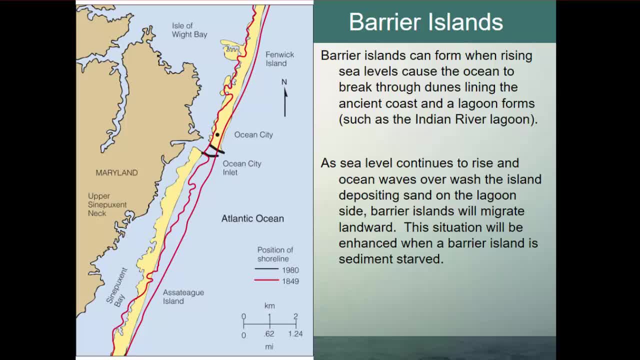 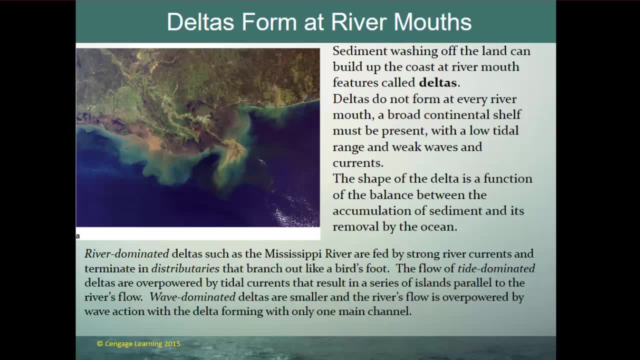 and um. essentially it caused that that island to migrate westward all right. deltas, like the mississippi river delta sediment washing off the land can build up the coast at river mouth and these features are called deltas. deltas do not form in every river, that is, in the ocean or river, but they do form in the ocean. so you can see the difference in the 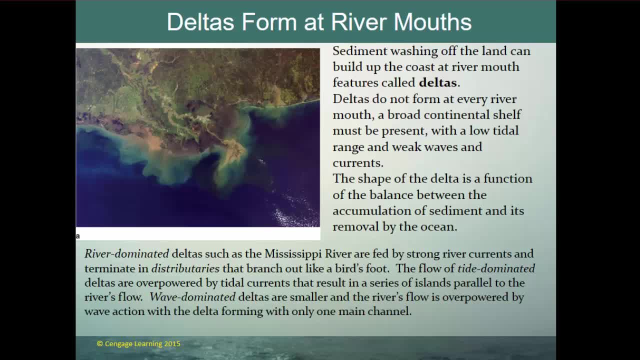 cooling effects of sediment and in order to get sediment from the ocean and out of the ocean, when you open a big, big, wide continental shelf, you have to have a continental shelf, a broad continental shelf present, with a low tidal range, meaning not a lot of water moving back and forth. 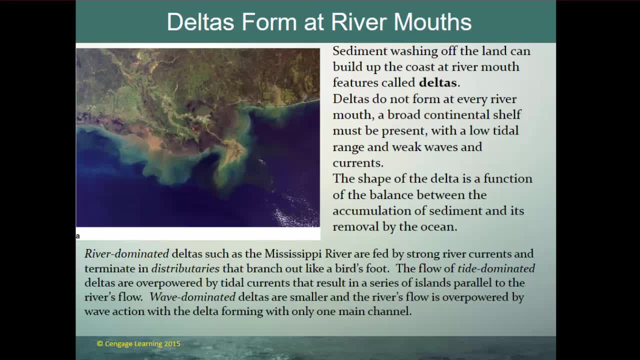 and weak waves, because if you have a lot of water moving back and forth in big, huge waves, all that sediment is going to just get washed away. but where you have a broad continental shelf, low tidal range and weak waves, you're going to get a big delta forming. 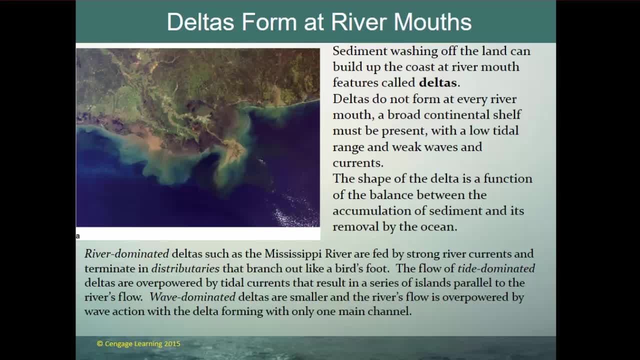 Different situations create different delta shapes, So river-dominated deltas such as the Mississippi River are fed by strong river currents that terminate in what are known as distributaries- You've probably heard the term tributary. A tributary river is the smaller rivers. 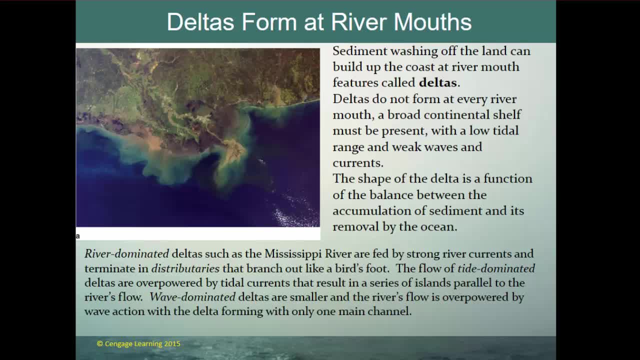 that feed the larger river. So a distributary is when a larger river feeds the ocean when it comes to its terminus, And the distributaries tend to branch out like a bird's foot and you get those deltas that we think of like a triangle. 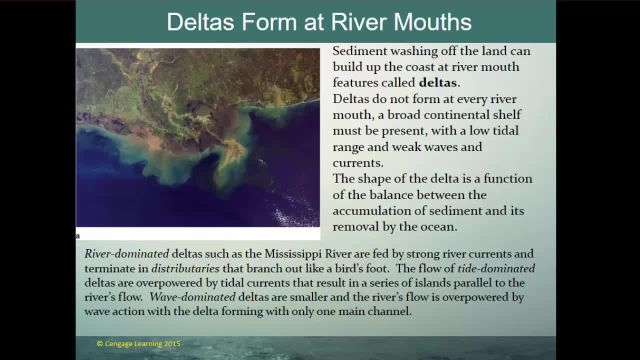 And those are river-dominated deltas. A tide-dominated delta is when tidal currents literally overpower the river and move inland. So the Mississippi River is always flowing south, but in a tide-dominated river the tide actually pushes up the river And that typically results in a series of islands. 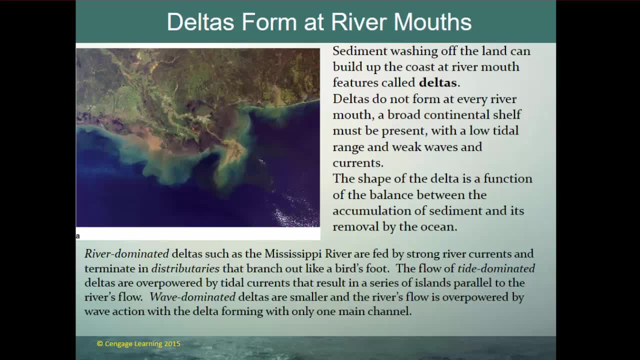 that are parallel to the river flow. Wave-dominated deltas are smaller, where the river flow is overpowered by wave action and you only get one main channel. So three basic different types of deltas And of course the Mississippi River is going to be that river-dominated. 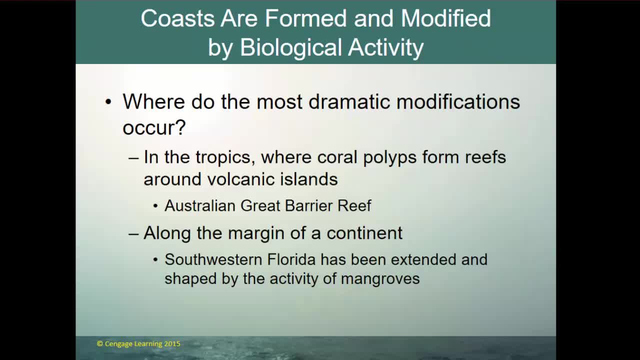 bird's-foot type of delta that's actually in the shape of a triangle. So coasts are formed and modified by biological activity as well. Lots of processes go into forming and modifying the coast. One of those processes is going to be biological activity. 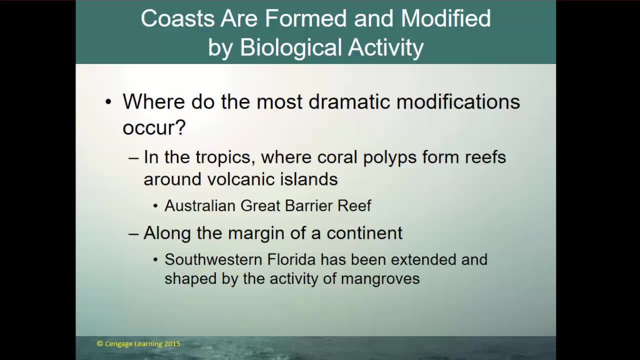 So where do we find the most dramatic modifications? In the tropics, where corals grow. Coral polyps grow and they form reefs around volcanic islands. So the volcanic island, the volcano pokes up under the sea and suddenly you have land above sea. 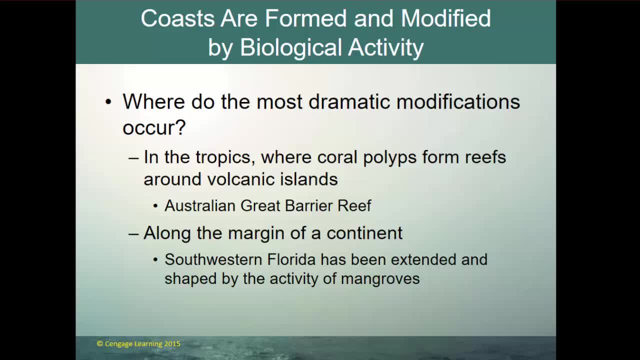 And then, over time, corals will develop what are known as fringing reefs around that island and you get these coastlines, these new coastlines that are created. So you have them created around islands, but you also have biologic activity around the margin of a continent. 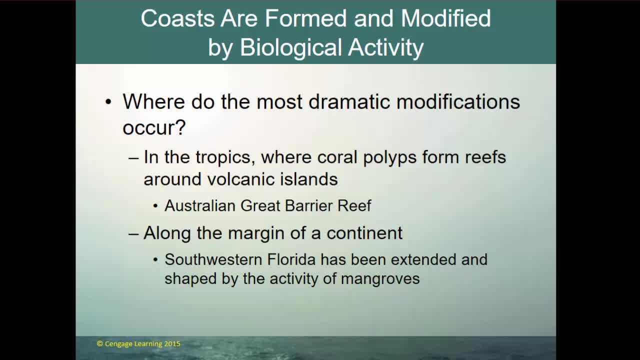 Southwestern Florida has been extended and shaped by the activity of mangroves, where mangroves are plants that can grow in brackish water and, as they grow out, their roots hold sediment and sand in and the land literally moves out with the mangroves. 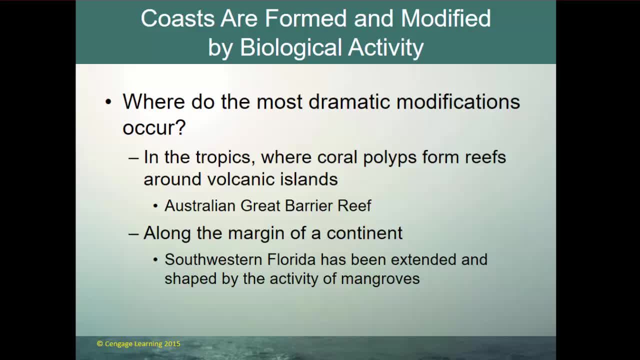 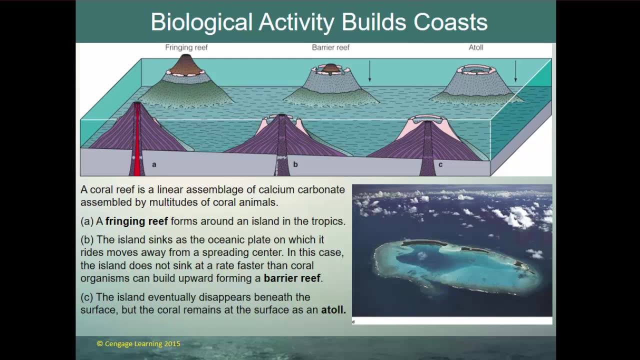 And so the coastline has been shaped by that, and the mangroves as they go further and further out extend that. So biologic activity in lots of different ways can help to form a coastline. So here's the example of the fringing reef. 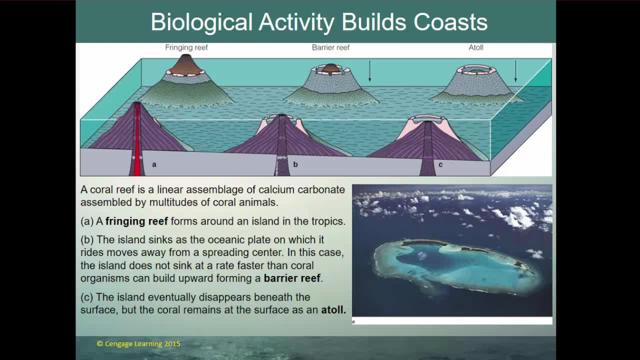 So you've got your little island that has popped up, and you have your fringing reef, and then, as that island begins to be eroded away and be, what you get is an atoll oftentimes. Well, an atoll forms eventually. 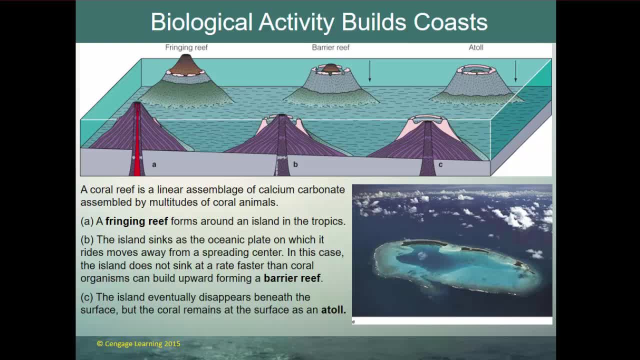 You get a barrier reef which is around the smaller island, and then, once that island is completely eroded away, then you get your atoll. So a coral reef is a linear assemblage of calcium carbonate created by multitudes of corals. 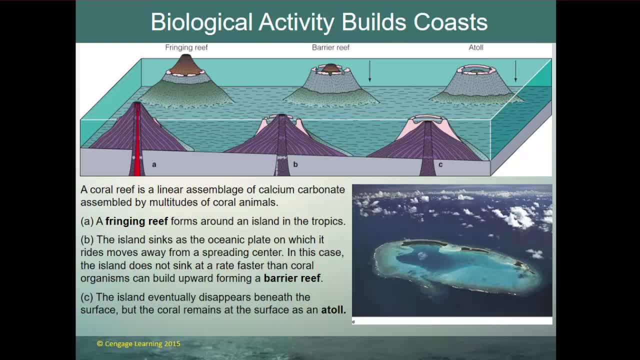 So corals are the individual little polyp animals. they create the calcium carbonate shell around them and that's the actual coral. So first you get the corals right along the coastline, that's going to be your fringing reef As the island sinks. 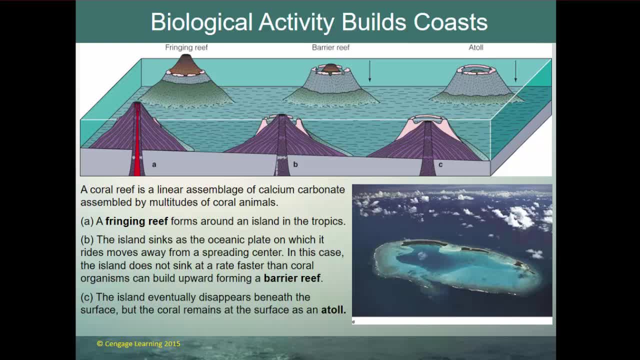 and that's largely from erosion, but also, as we talked about, in tectonics. the ocean plate on which it rides is moving away from the spreading center, and so it's getting deeper and deeper. Remember, the mid-ocean ridge is at a higher. 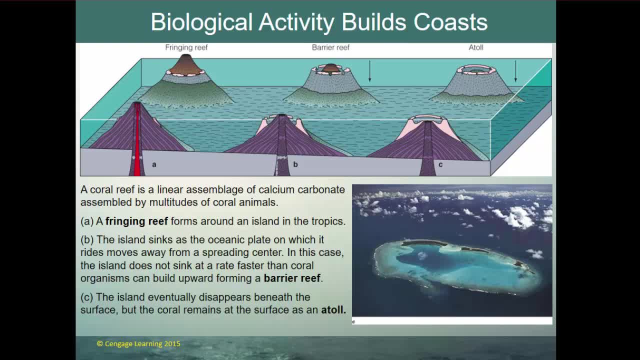 let's say seafloor elevation. and as it moves away it gets deeper and deeper. So these volcanoes that are formed close to the mid-ocean ridge, they will eventually sink, and as they sink they get lower and lower. 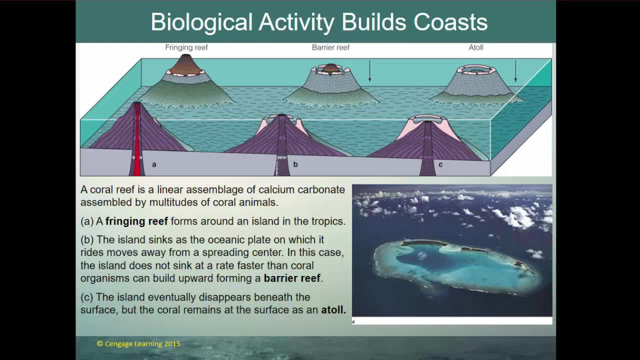 but as you can see in B, the coral reef just gets higher and higher. It grows up toward the sunlight, so it continues to get higher and higher and so eventually you get these atolls. So in the case where the island does not sink, 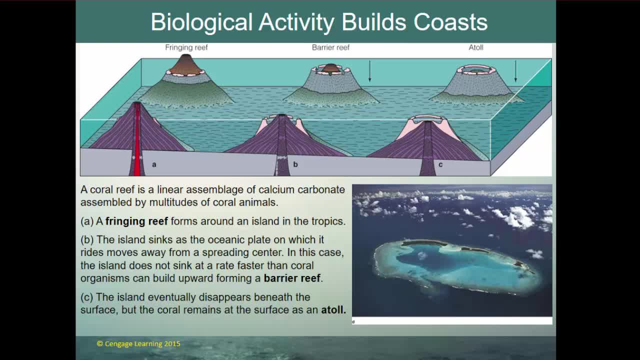 at a rate faster than the coral organisms can build. you get a barrier reef, but eventually the island will disappear beneath the surface. but the coral remains at the surface and that's where you get your atoll, And that little picture at the bottom right is an atoll. 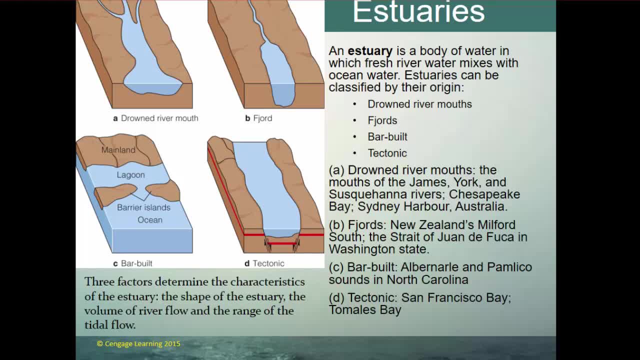 All right, now I'm going to talk about estuaries, and estuaries are very important: the location of tremendous amounts of biologic activity. An estuary is a body of water in which fresh water mixes with ocean water, and estuaries can be classified by their origin. 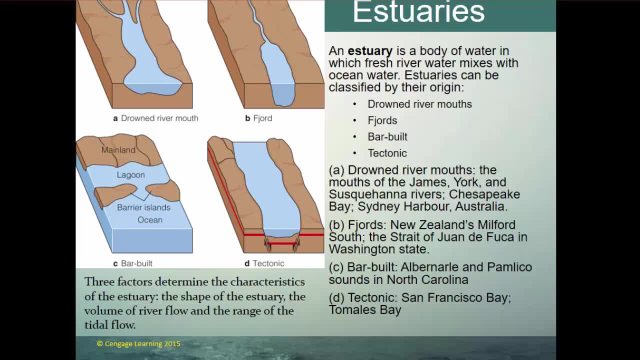 We have drowned river mouth estuaries with fjords. We have bar-built estuaries, tectonic estuaries, so drowned river mouths like the mouth of the James, the York and the Susquehanna Rivers, the Chesapeake Bay, Sydney Harbor in Australia. 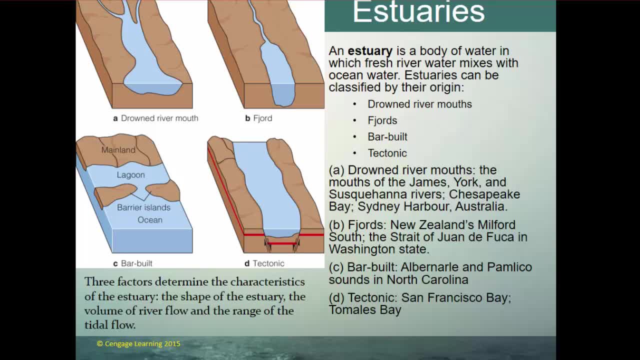 those estuaries are where river mouths have been drowned by a rise in sea level, Fjords like in New Zealand, and also in the northwest coast of North America, in Washington State, the Strait of Juan de Fuca. they are again where those deep channels 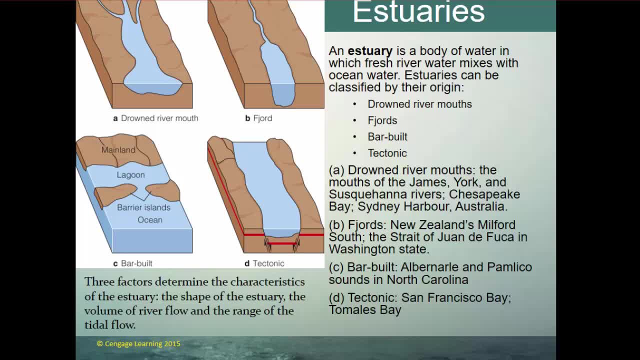 are flooded out as sea level rises and you get those very, very deep U-shaped estuaries. and again the U-shape has come by some previous glacial advance that carves out that U-shaped channel Bar-built, like the Albemarle and Pamlico Sounds. 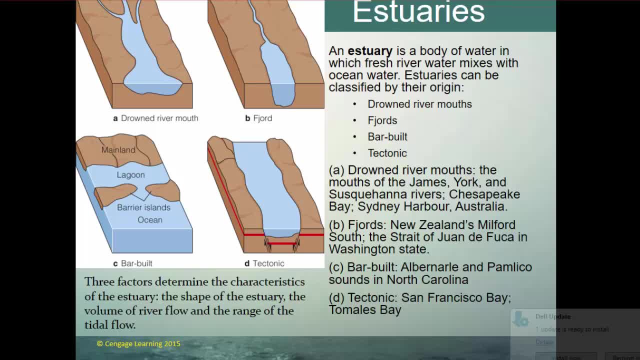 are North Carolina, where you get barrier islands and then the lagoon behind them becomes has lower salinity because fresh water flows, and then tectonic, like San Francisco Bay, where some down drop because of tectonics. and so if we look at this, 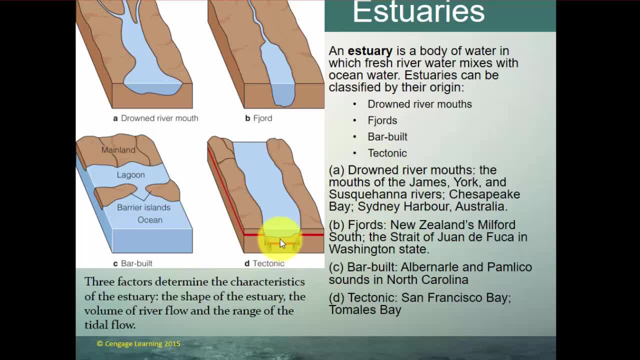 this is a situation where we have a divergent coastline, so the red line shows where everything was at one time, but plates are moving apart, so that plate's moving in that direction. this plate's moving in that direction and it causes this to fall, to sink down. 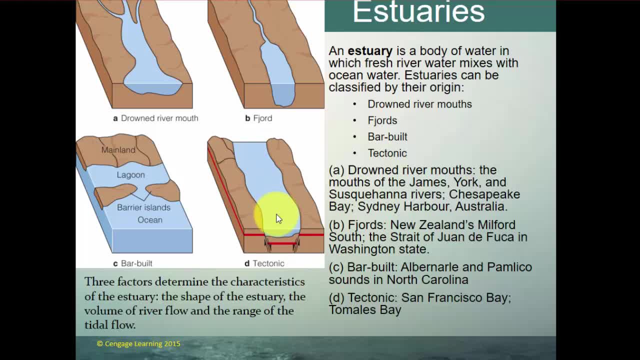 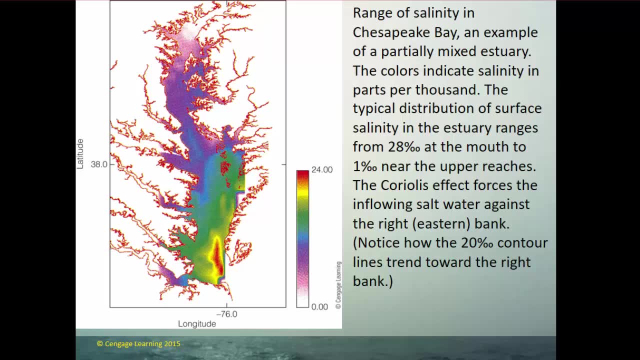 and that creates a bay or an estuary like what we see in San Francisco Bay. All right, so this is the range of salinity. So the white is where there's fresh water and the red is where it's saline, and this is gonna be the Chesapeake Bay. 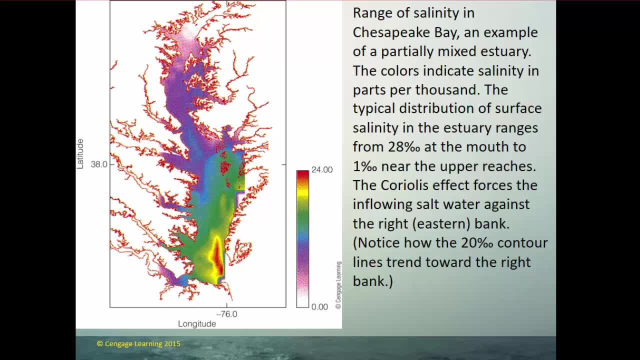 where these tributaries feed the bay with fresh water and you can see how the salinity increases as you get closer and closer to the ocean. So it's an example of a partially mixed estuary. The colors indicate salinity in parts per thousand. 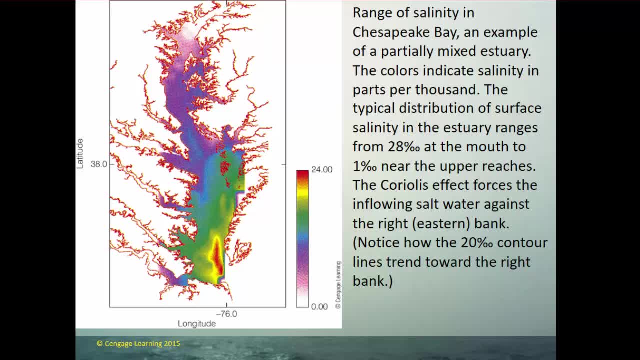 The typical distribution of surface salinity in an estuary range is some 28%. You can see the salinity in parts per thousand in the upper reaches of the estuary. So you can see something interesting: The Coriolis effect or the movement. 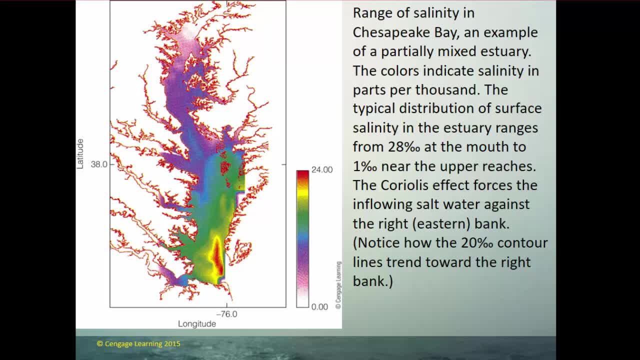 in the northern hemisphere to the right forces the inflowing saltwater against the right or the eastern bank and so that higher stripe of 20% contour tends toward the right side of the bank. But that is a partially mixed estuary where fresh water flows in. 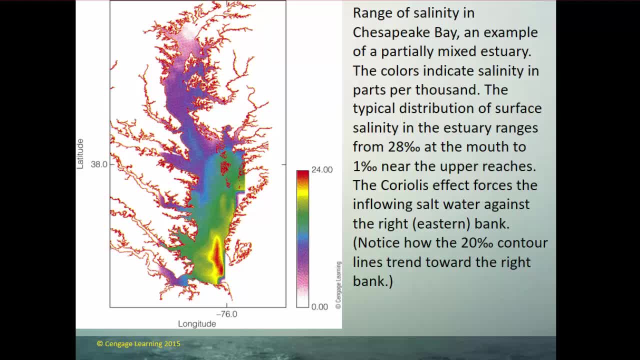 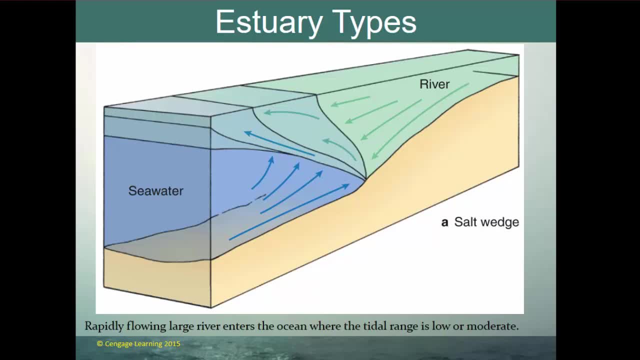 and then tidal push pushes saltwater in from the mouth, So we'll have a couple different types of estuaries and we'll see cutaways of each one. A rapidly flowing large river basically keeps the ocean at bay, and the ocean seawater is going to be denser. 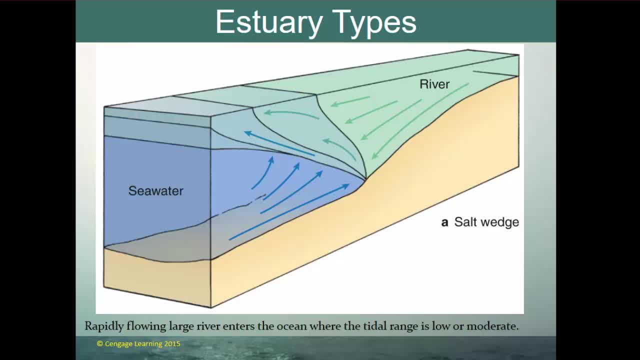 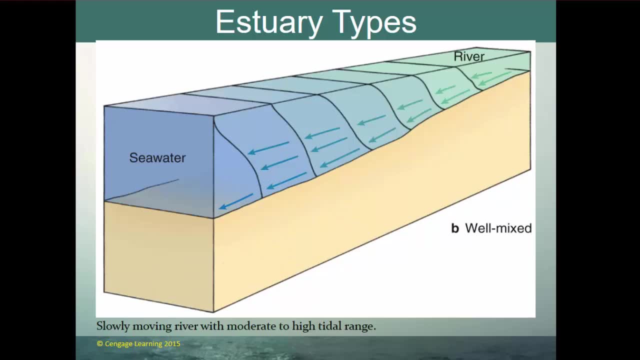 so it's gonna sink, and so you're gonna get this wedge where fresh water lies on top of saltwater, and so this is called a salt wedge estuary. And then you have a well-mixed estuary where slow-moving rivers with moderate to high tide. 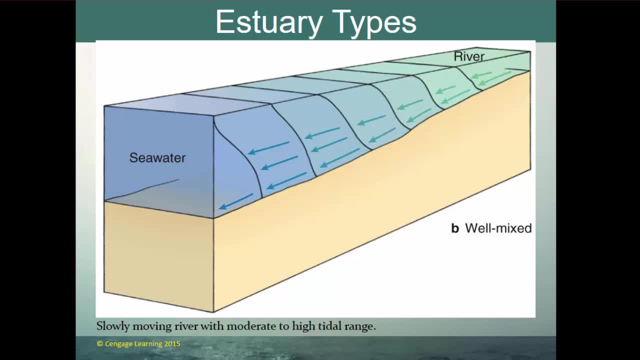 moderate to high tidal range. so the high tidal range means that as the tide goes high, it pushes saltwater in, and as the tide goes low, the slow-moving river pushes fresh water out and you get this well-mixed estuary. 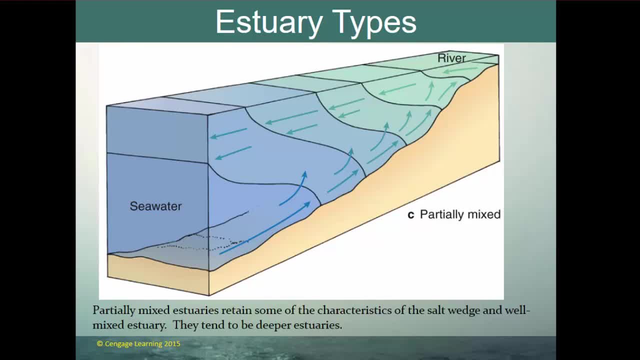 And then you get a partially mixed estuary like the Chesapeake, and a partially mixed estuary retains some of the characteristics of a salt wedge and some of the characteristics of a well-mixed. It's somewhere in between, and they tend to be slightly deeper estuaries. 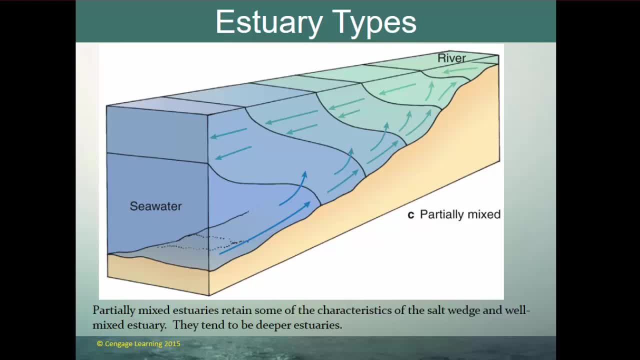 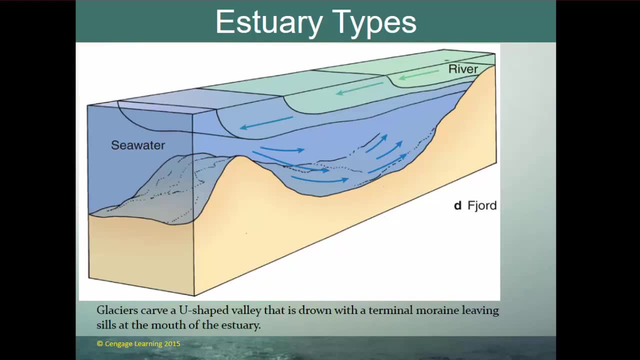 and you can see there's still a little bit of a salt wedge, but there's also some mixing that goes on as well. And then we have the fjord, and again in the fjord, the glacier carves out this U-shaped valley. 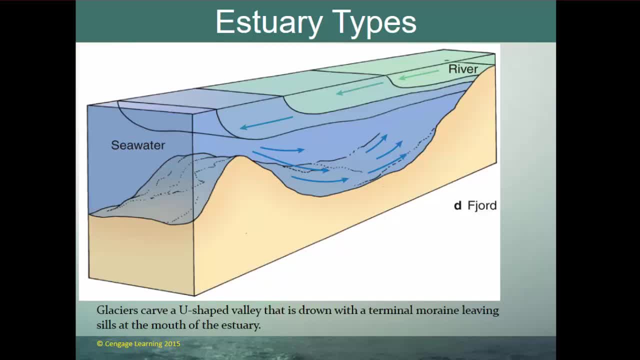 but when glaciers form they get to a point. they get to a certain point and at that end point where they stop eventually, when they recede, they dump a tremendous amount of sediment at that end point and those mounds of sediment are known as moraines. 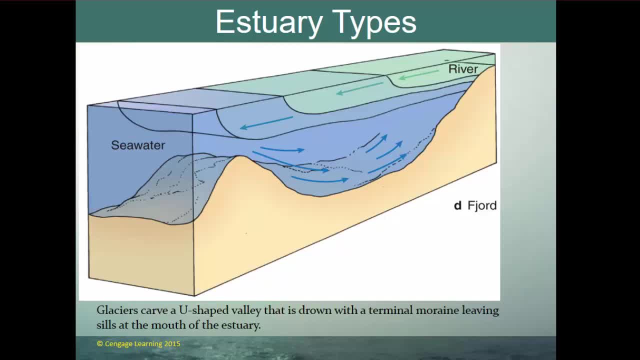 and a terminal moraine is the furthest extent of the of the glacier and they also leave other moraines back as the glacier retreats, but the terminal moraine is this last one. So as a glacier, an alpine glacier, comes down a valley. 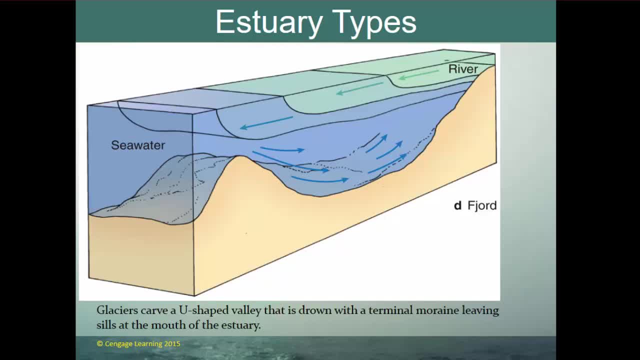 and carves out this U-shape, it gets to a point where it stops. that's where it leaves the terminal moraine, and that terminal moraine acts as a sill at the mouth of the estuary and it creates this estuary type, this fjord estuary. 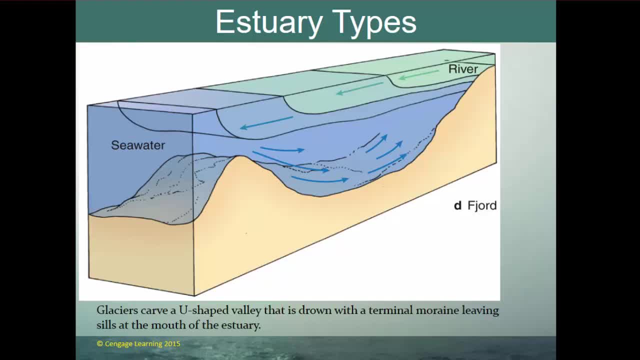 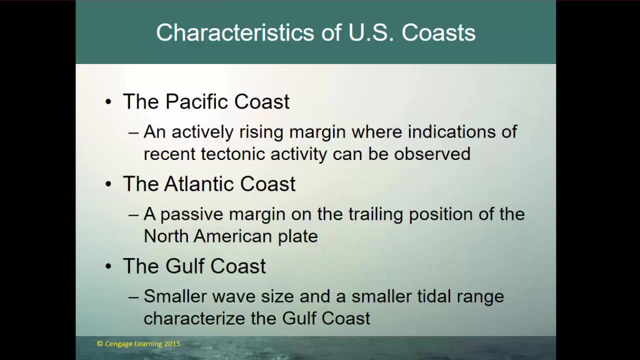 where you have this layer of freshwater on the top and a layer of saltwater on the bottom. So what are the characteristics of the US coastline? Something that we should all be able to identify with. The Pacific coast is an actively rising margin. 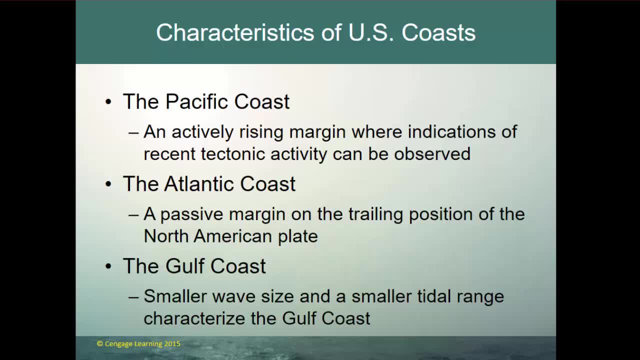 where indications of recent tectonic activity can be observed. It's an emergent coastline, alright. The Atlantic coast is a passive margin on the trailing position of the North American plate, so the North American plate is moving off to the north and west. 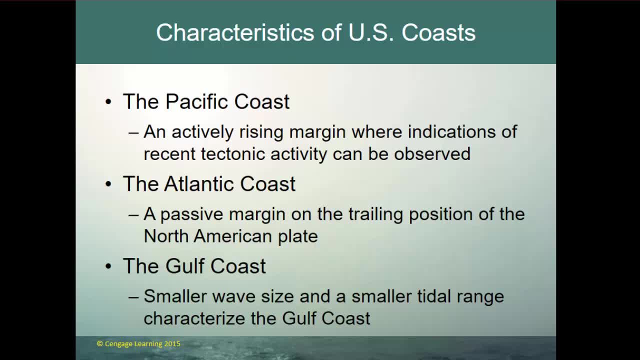 and we're on the southeast corner of it, in the Atlantic coast, the eastern corner of it, so we're on the trailing portion of it, so it's a passive margin. And then the Gulf coast is this enclosed basin, which means it has smaller wave size. 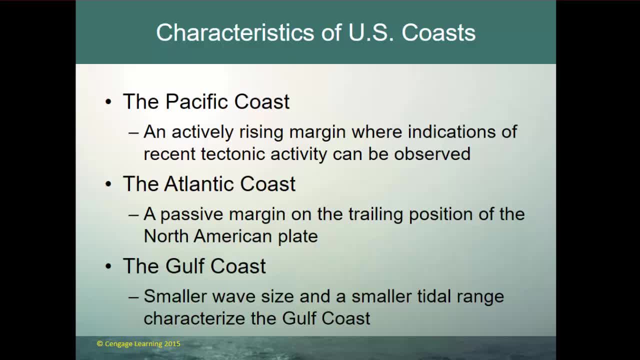 but also smaller tidal range, and that's what we get with the Gulf coast And also on the Atlantic coast you tend to get two high tides, two low tides a day, but if you're on the Gulf coast you only get one. 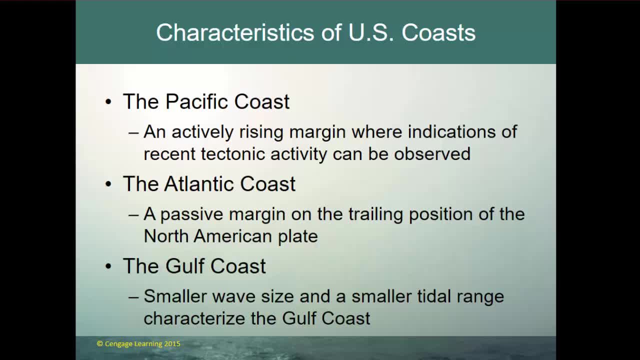 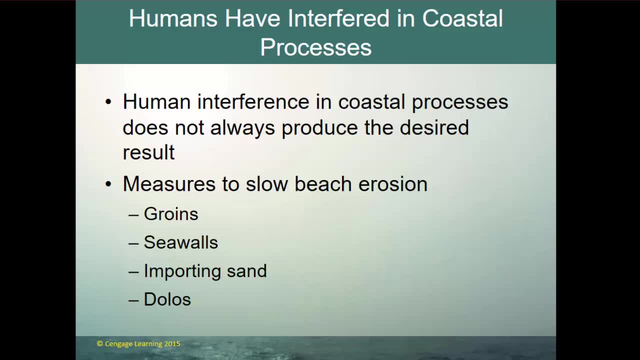 and that's again because it's that smaller, enclosed basin. The water tends to slosh sort of back and forth over 24 hours in that basin. So humans certainly interfere in coastal processes. Human interference in coastal processes does not always, however, result in the desired. 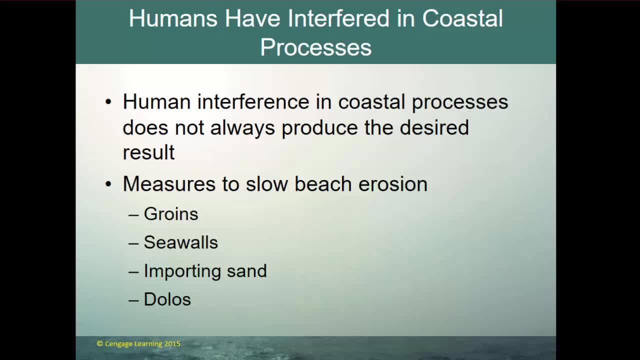 well, the desired result is the law of unintended consequences. Oftentimes, human interference is meant to slow beach erosion. You build a $200 million fabulous resort on a beach and then next year big waves come and wash the beach away. 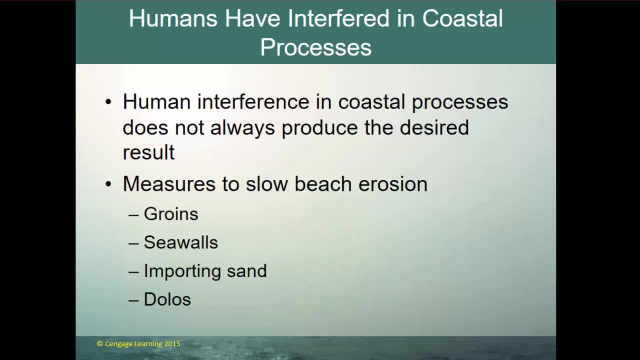 Your visitors don't like that. So what do you do? You build a seawall or you build a groin or you build any other types of structures that can potentially help to hold your sediment in, hold your sand in like a jetty. 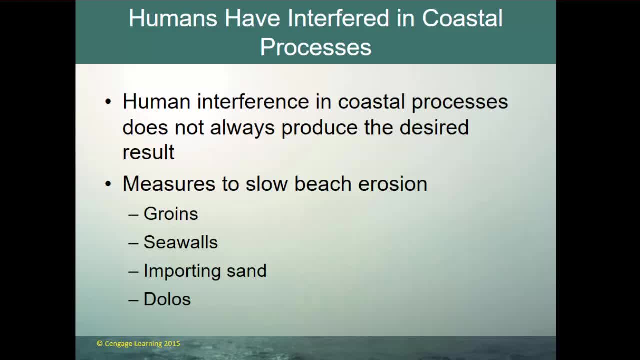 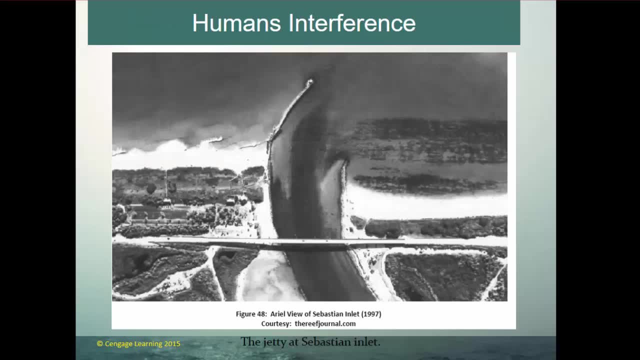 Unfortunately, those types of structures tend to starve other areas of the coastline of that sand. So here is a view of Sebastian Inlet with a Sebastian jetty on the north side, and of course the longshore current tends to be from north to south. 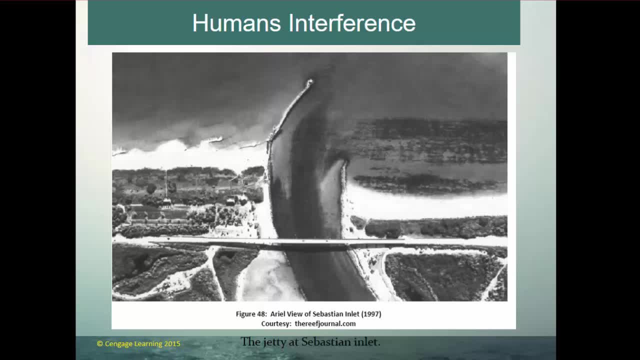 It goes along the east coast of Florida, and the large, long jetty on the north side slows the water down and causes the water to largely dump its sediment on the north side, And so you can see how the beach has literally receded on the south side because it is sediment starved. 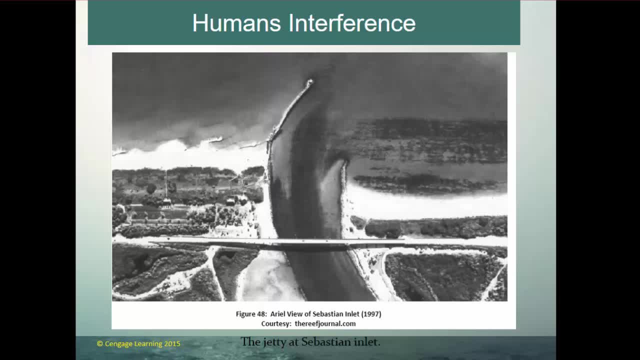 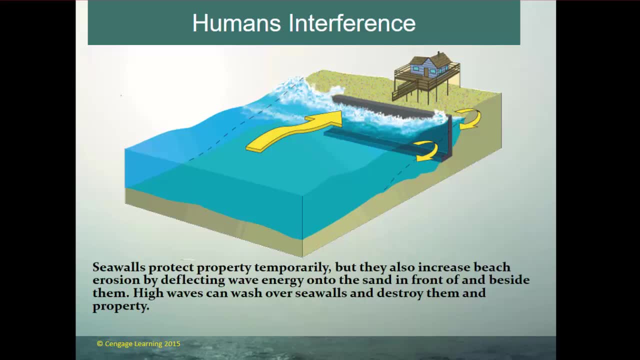 and it's sediment starved by that jetty. So the jetty is very, very good at saving the sand on the north side, but it causes a problem on the south side. So seawalls tend to protect property temporarily, but they also increase beach erosion. 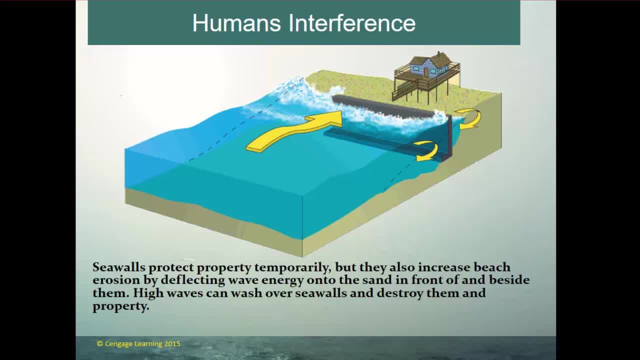 by deflecting wave energy onto the sand in front of and beside the seawall. So you take any sand that was in front of the seawall away, so that's just exposed seawall, and then on either side of the seawall the waves are focused. 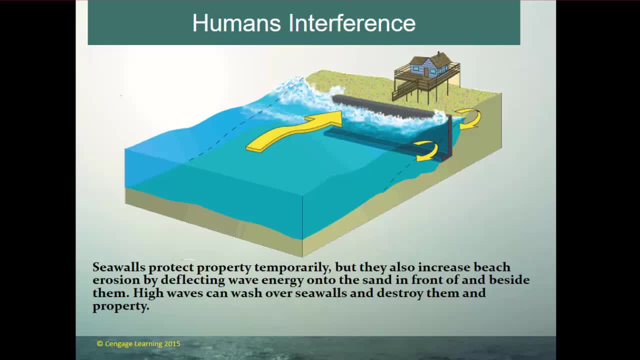 and you pull sand away from that area. So it's fine for the house on stilts, but it's not good for the water out in front of the house and it's not good for the beaches on either side of the house Also. high waves can then wash over the seawall. 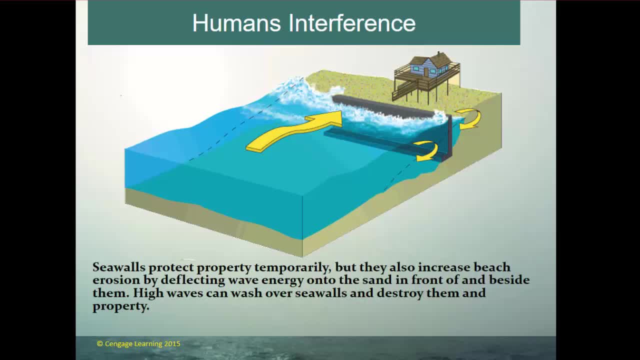 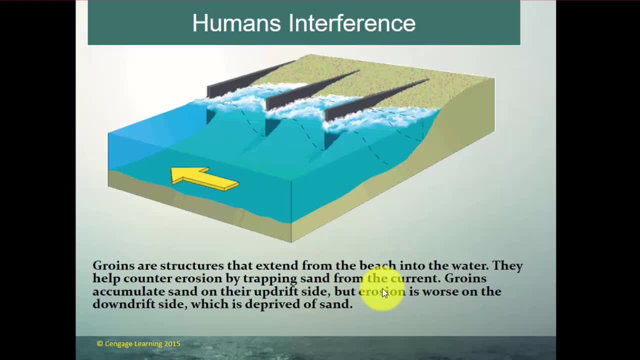 and destroy them, and then the water still gets to the property and you've also destroyed the beach lines. Now, groins are structures that are built perpendicular to the wave action, but they have the same effect as a jetty And oftentimes 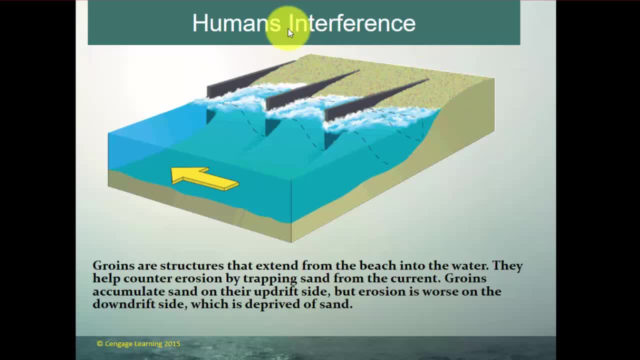 and you see a lot of this in South Florida, where you have one luxury hotel after the other. each hotel right on its southern edge will build a groin and you can see how that groin holds sand on the north side and then depletes sand on the south side. 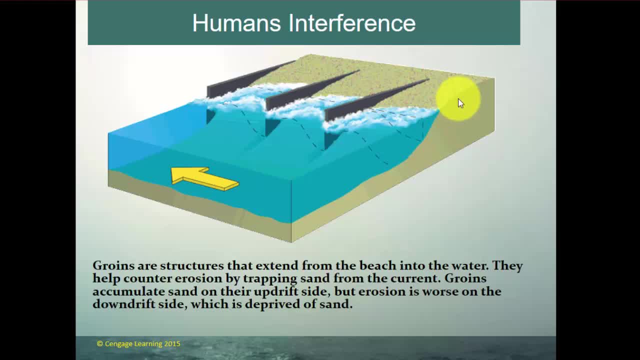 So if you built your hotel here, you build a groin, you keep your beach. but the guy who builds a hotel here, he loses his beach, so he builds a groin. So it's a process they do right down the beach. So groins are structures. 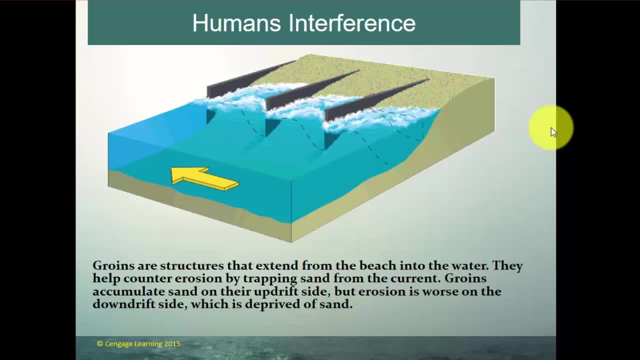 that extend from the beach into the water. They help counter erosion by trapping sand from. the current Groins accumulate sand on their up-drift side, but erosion is worse on the down-drift side, which is then deprived of sand. So groins are good for people who build them. 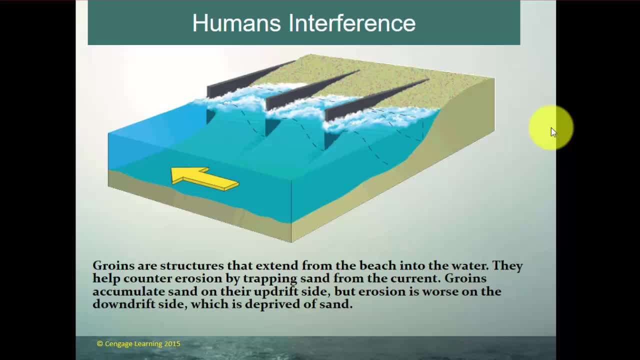 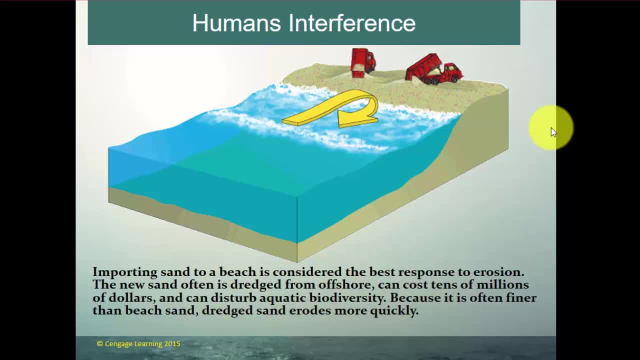 but not good for people down-drift of the groin itself. The other thing that humans do is they import sand onto beaches, and it's considered to be one of the best responses to erosion. However, of course, eventually that sand is just going to be eroded away. 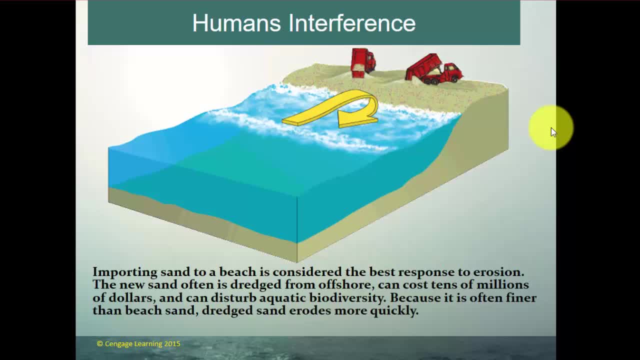 New sand is oftentimes dredged from offshore, so the quality of the sand is not the same as the sand that was naturally there. The sand that's naturally there is going to be more well-sorted. It's going to be typically cleaner. 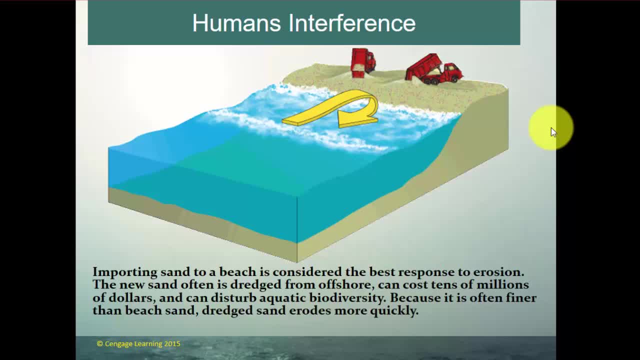 and also this can cost tens of millions of dollars. It can disturb aquatic biodiversity, and then oftentimes it's going to be finer because you get more siltier types of sediments offshore, which also makes it dirtier, and so it's more easily eroded. 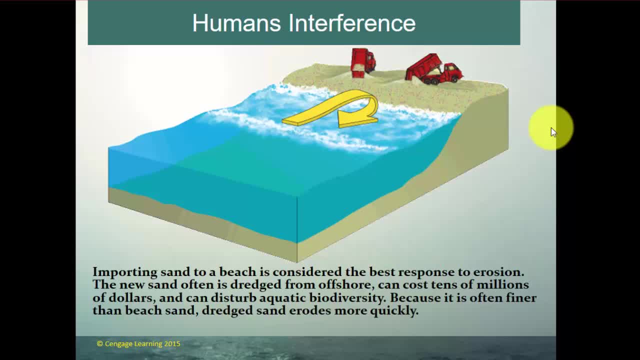 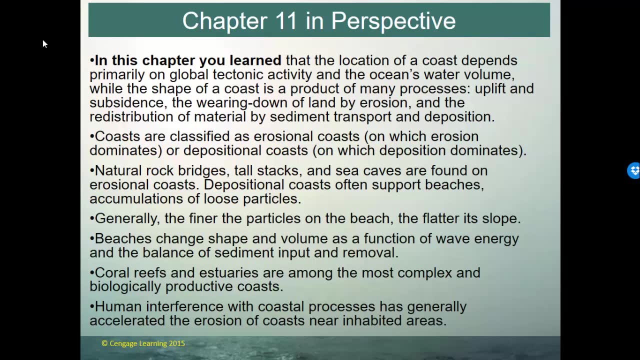 So you know, it's easy to see it work. You bring the sand in and it works and you have a new beach, but then it gets eroded almost more quickly than the previous beach. In Chapter 11, we've learned that the location of a coast 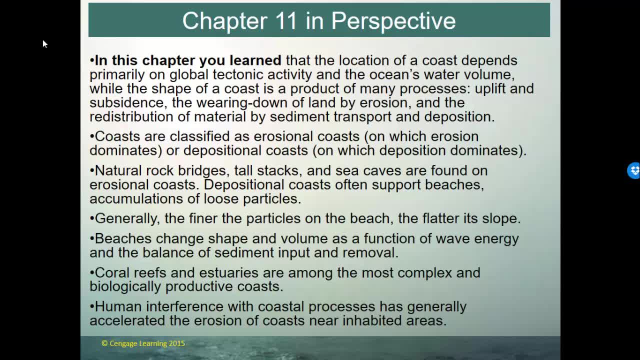 depends primarily on the global tectonic activity and the ocean's water volume, while the shape of the coast is a product of many processes: uplift and subsidence, erosion, redistribution of material by sediment, transport and deposition. even the biological activities of creatures along the coastline. 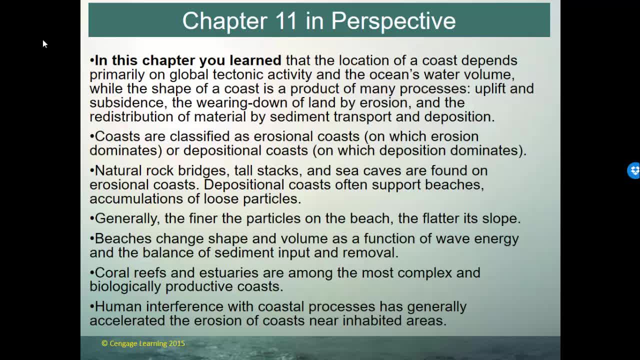 Coasts are classified as erosional, on which erosion dominates, or depositional, on which deposition dominates. Natural rock bridges, tall stacks, sea caves are all found along erosional coasts. Depositional coasts often support beaches and accumulations of loose particles. 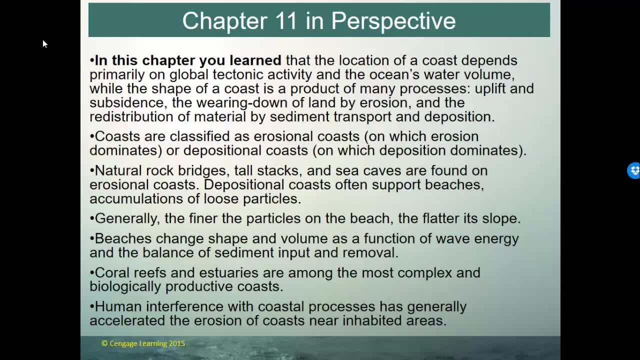 Generally, the finer the particle on the beach, the flatter the slope of the beach. Beaches change shape and volume as a function of wave energy and the balance of sediment input and removal, and coral reefs and estuaries are among the most complex.